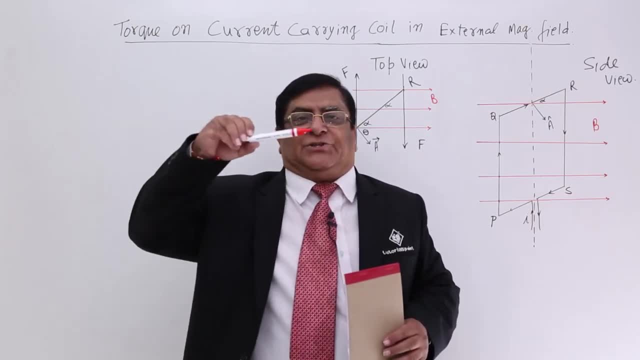 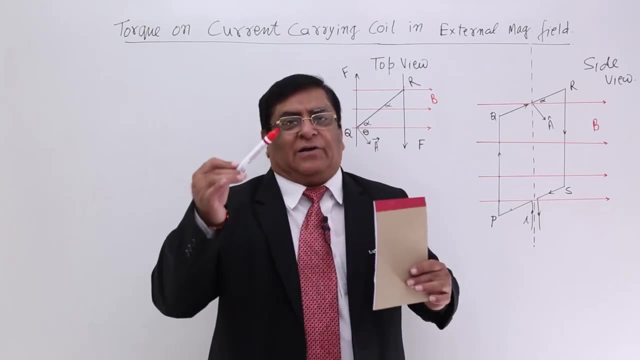 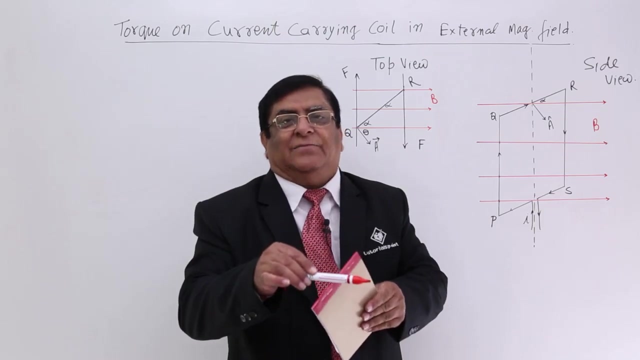 If there is a magnetic field, say, in this particular direction, and we place a coil here and flow current in it, For the sake of any general condition, I assume that they may not be parallel, they may not be perpendicular, They make certain angle, alpha with them. This is magnetic field. 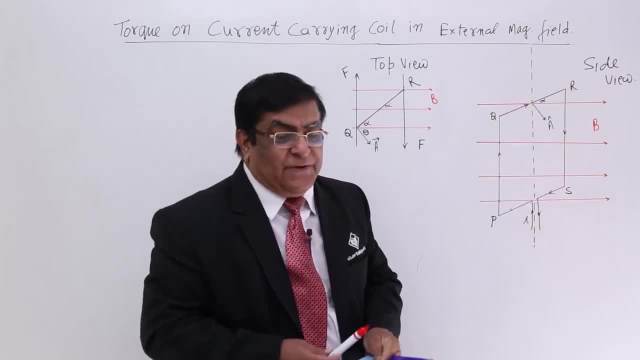 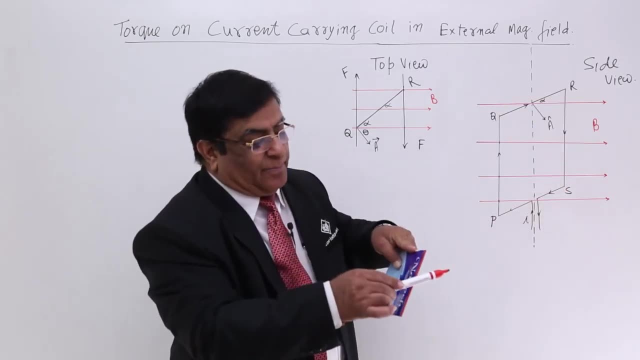 This is the coil position making angle alpha. If we see it from the side, as you are seeing it now, it will appear like this, But if you see it from the top, it will appear like this: This is the diagram top view and. 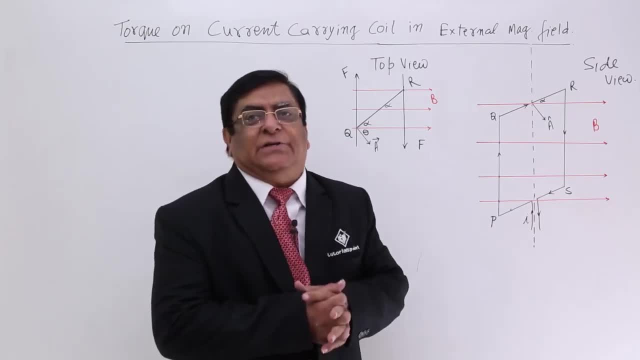 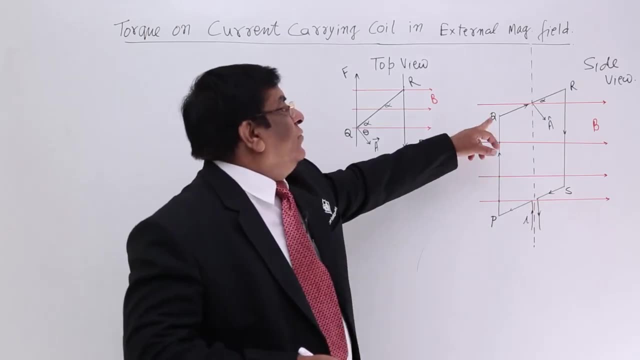 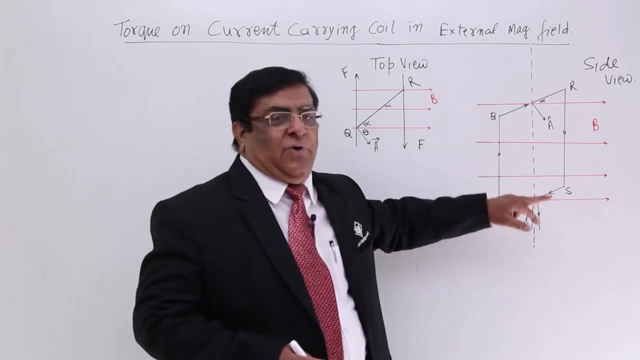 that is side view, So we have to understand both the ways, because in everything in magnetic we have to imagine three-dimensional diagrams. So we come here and the current flows in it. We will calculate two things. Number one: what is the force experienced by this coil? 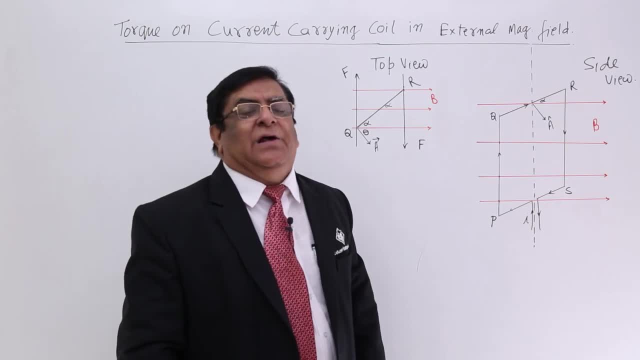 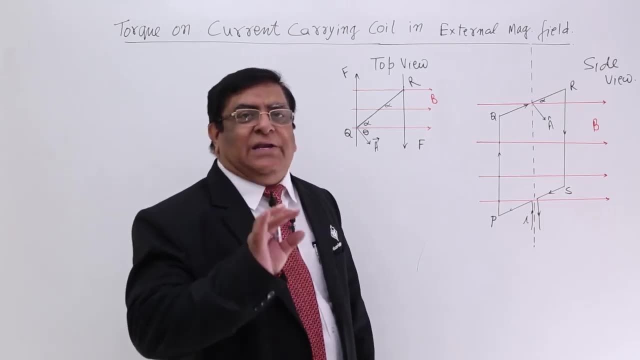 and number two: what is the torque experienced by this coil? Because we know that there are two types of motions: One is linear motion, one is circular motion. For linear motion, we need a force, For circular motion, we need a torque. So 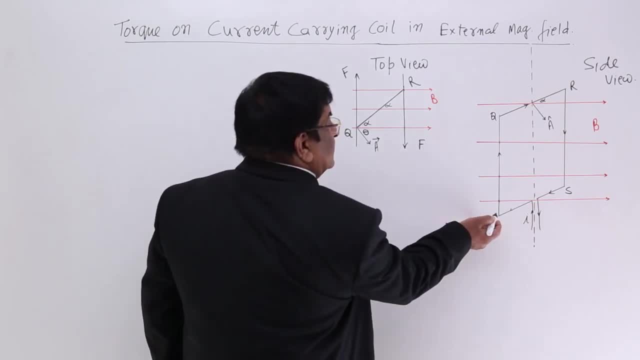 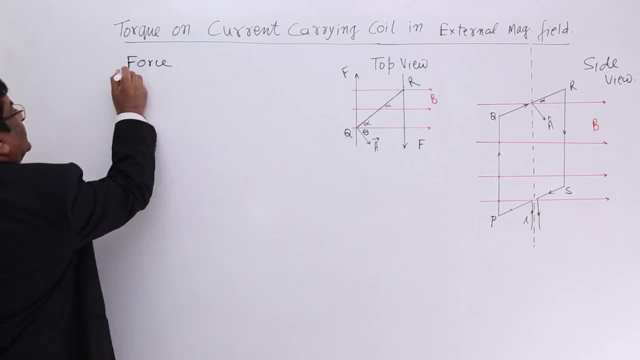 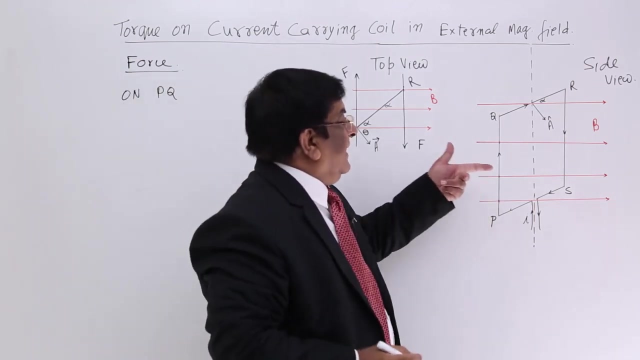 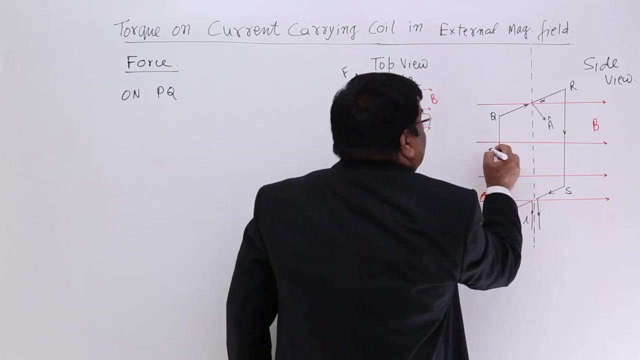 here. first we assume what is the force on PQ. We will calculate force first. Force on PQ. This is the magnetic field. This is the current. The force is inside. The force is inside here. This is the direction of force inside. I will make it as indicator of inside force Here. 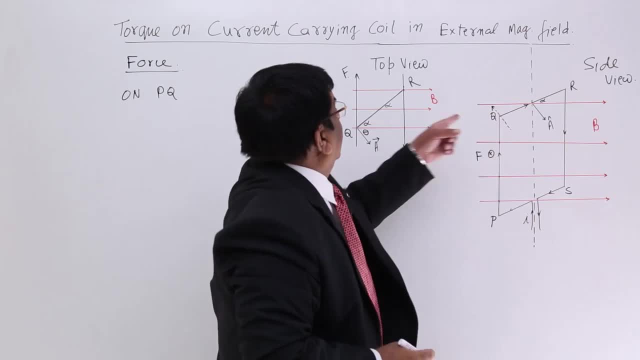 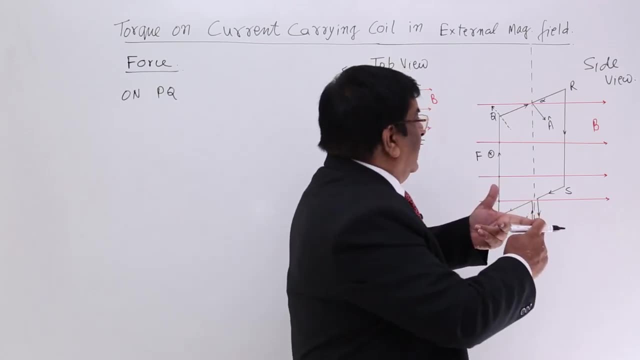 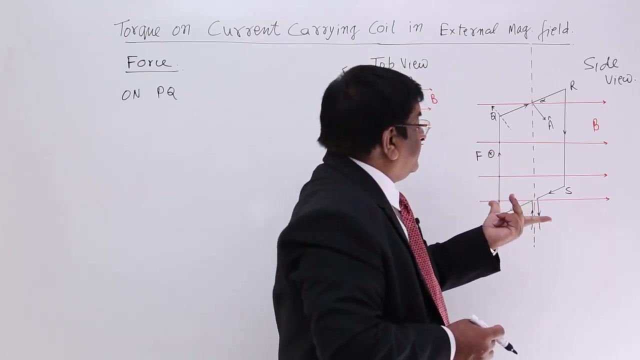 this is inside. force on PQ here. Now, force on this, This is magnetic field. This is the direction of force And this is the magnetic field. This is the direction of force inside And this is the ok. One portion of this which is perpendicular to it will make a force. 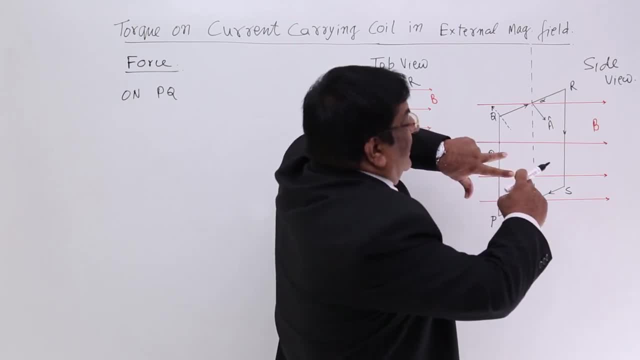 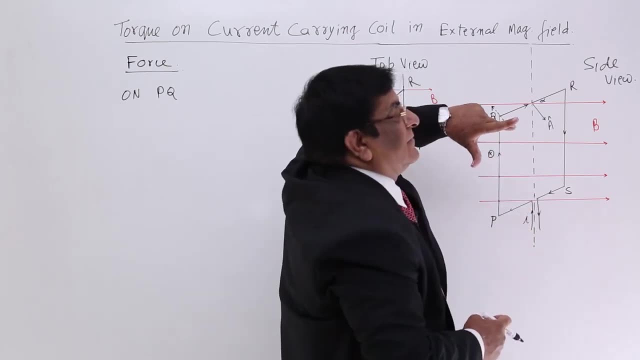 And what will. what is the plane of magnetic field and current? Answer: this is the plane of magnetic field and current, See Magnetic field and current. Then the force is always it. If the current has this direction, it has a component in this direction: magnetic. 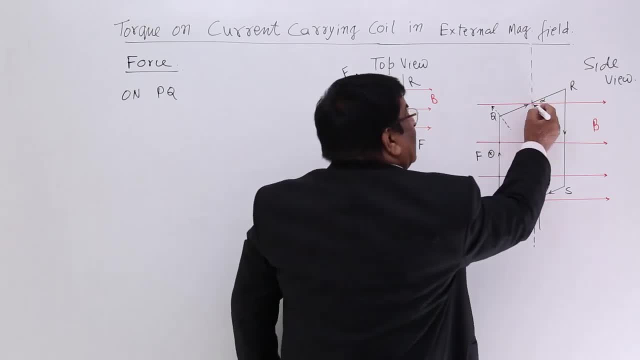 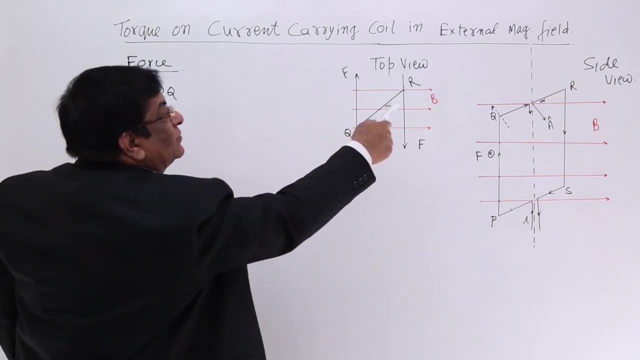 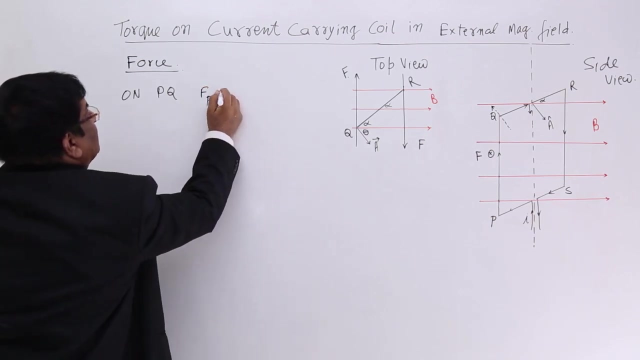 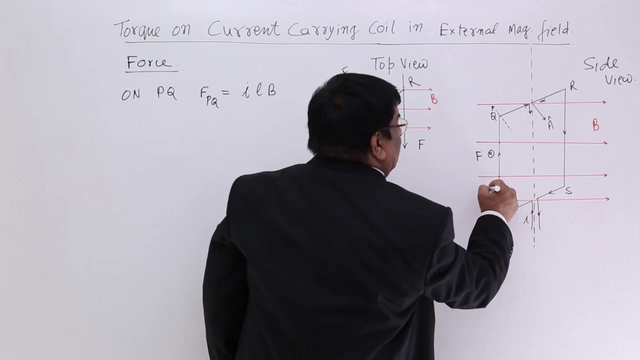 field in this direction, then the force is in this direction. So here we have a force acting downward, That is force on QR. So what is force on PQ? F on PQ, this is equal to i, into L, into B. i is current, flowing in it. Length of this conductor is L and B is the 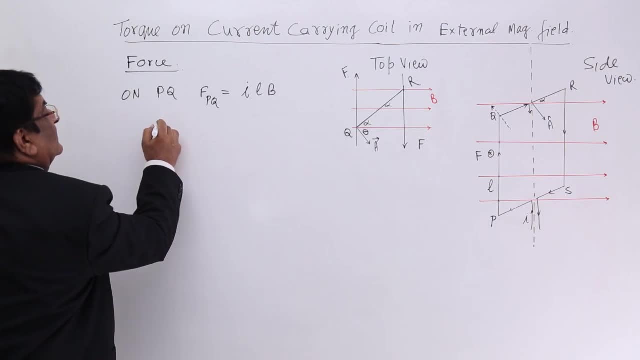 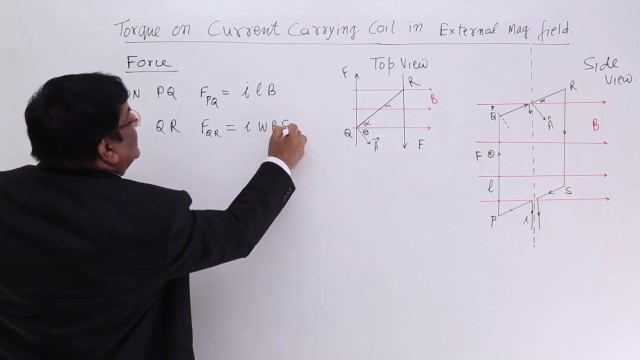 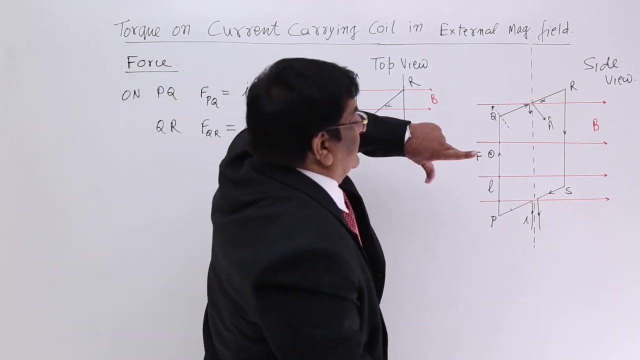 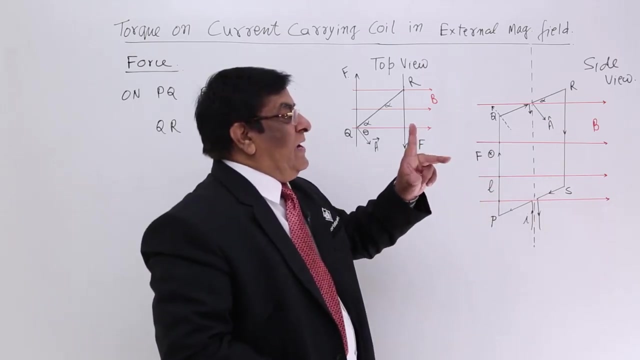 strength of magnetic field. Now, force on in place of PQ, we take as QR Force on QR. Force on QR is i into width, into B, into sin alpha. This is the force force and its direction is downward, downward. here it is sign 90, because this is up and 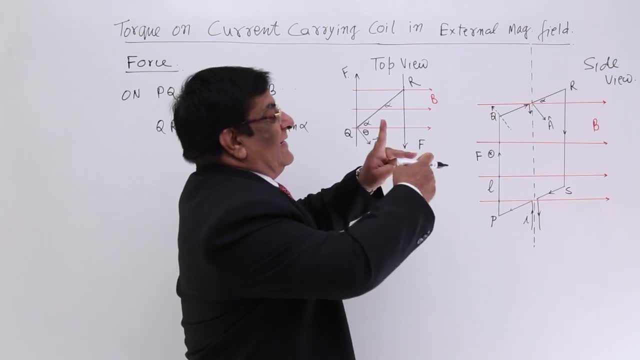 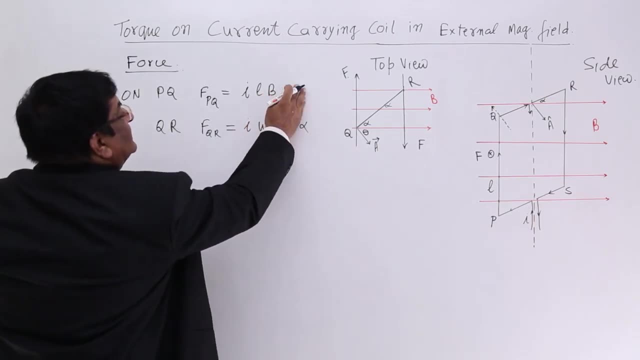 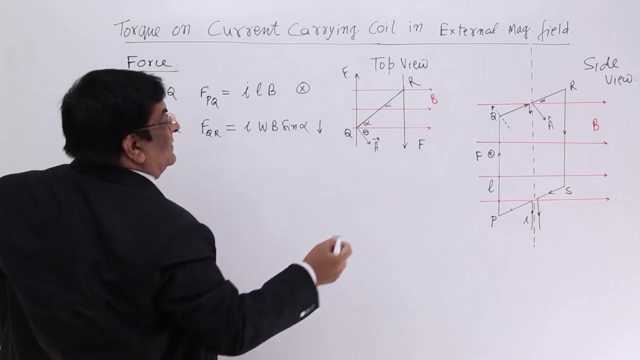 this is this way. this angle is exactly 90, but that is not in this case. in this case, it is only alpha. let it be. what will be its force direction? this is inside, so I will mark it here: inside. this is downward, I will mark it here now. force on third arm, that is RS. 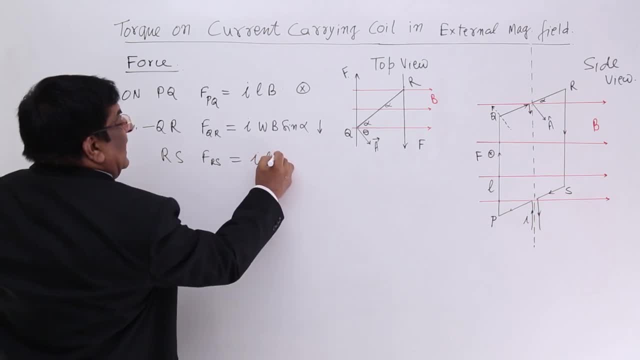 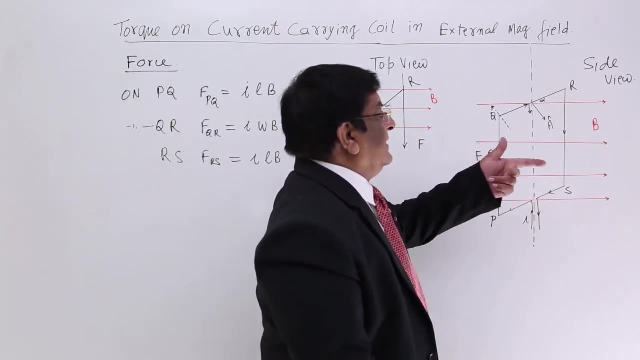 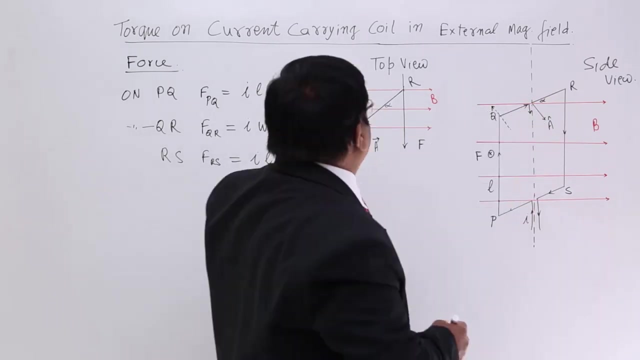 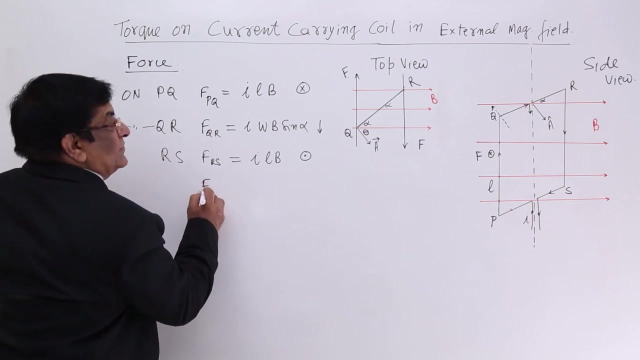 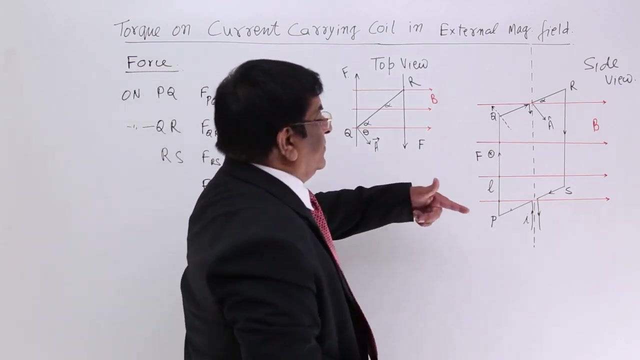 force on RS is equal to ILB and that is again sign 90. but what is the direction? here is the B and the current is going down. if the current is going down, the force is outward, and I will write it: the force outward, then force on SP. this force, this is the magnetic. 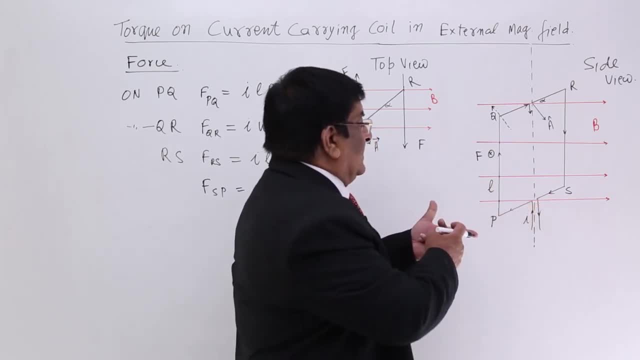 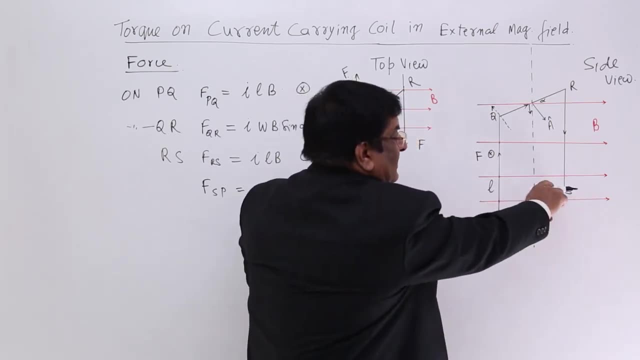 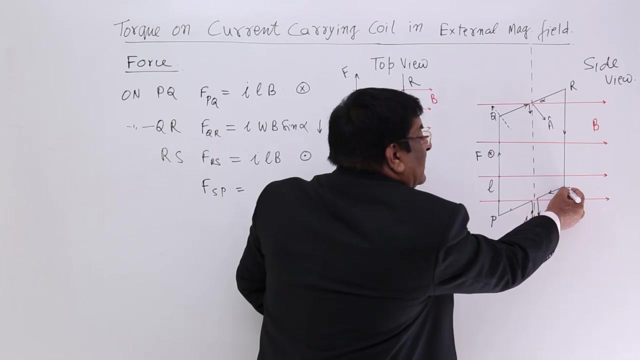 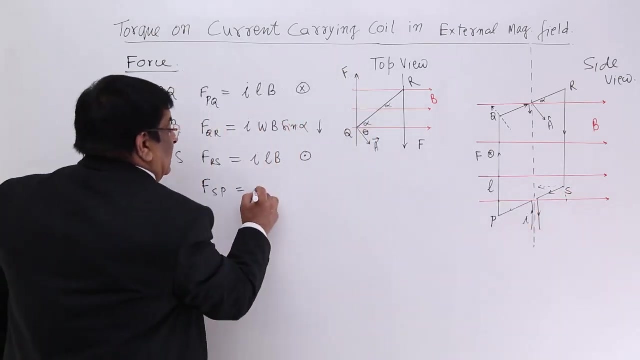 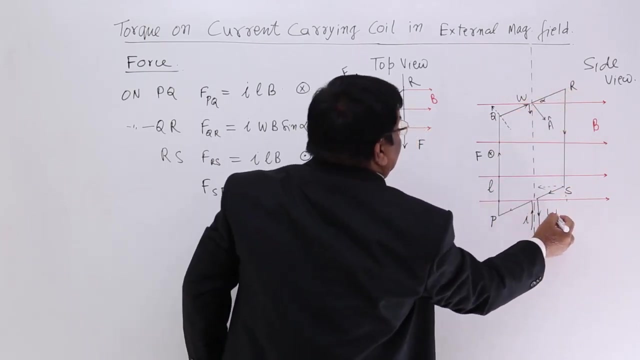 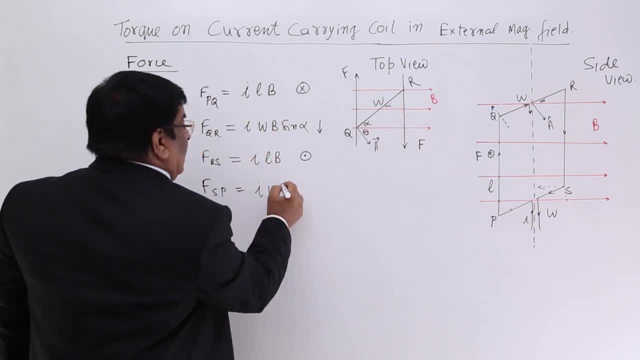 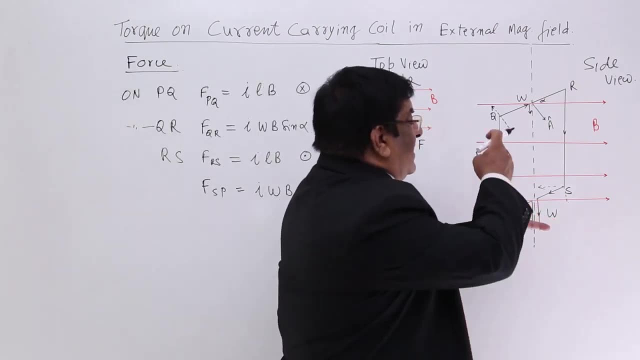 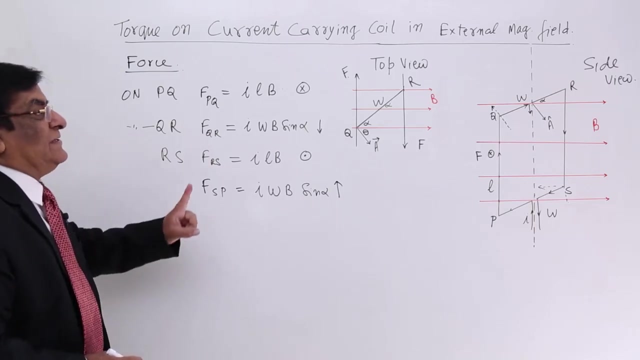 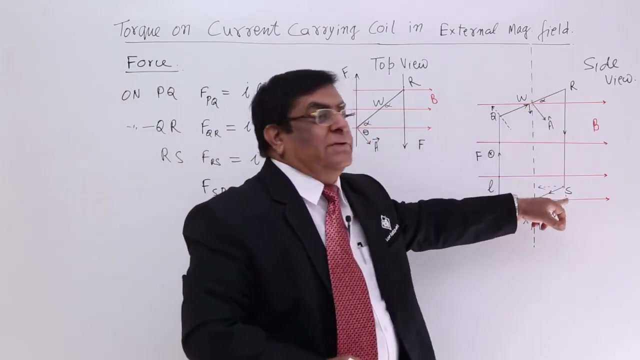 width. So this is IWB sin alpha. but its direction, see its direction. it is coming up, So this is going up. These are the 4 forces acting on the 4 straight conductors on it. Now, all these 4 conductors are bound to each other. they can apply force on each other. we cannot. 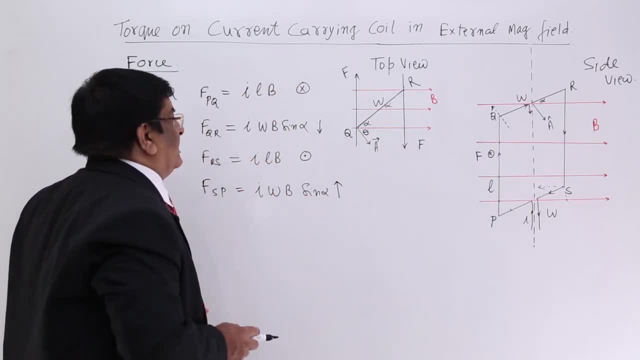 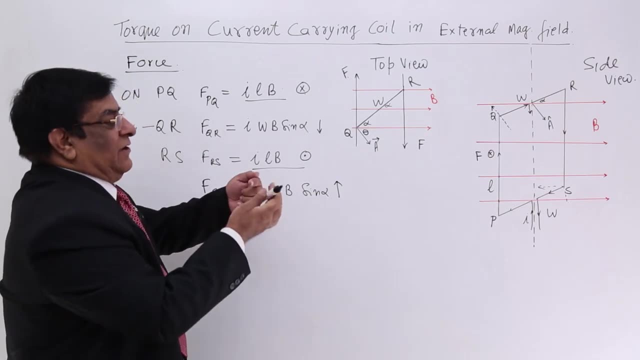 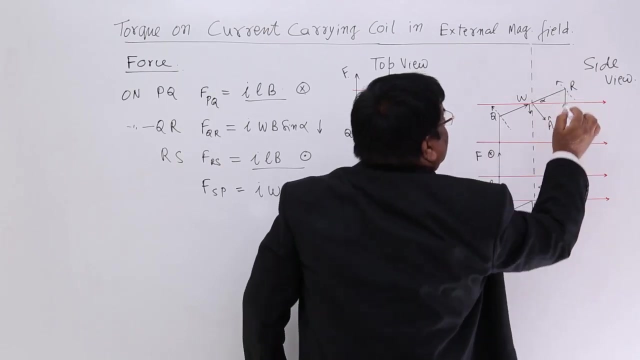 separate any one. Now see the forces, ILB inside, ILB outside, cancel each other. they are equal and opposite to the same body. Here, if it is working here, here it is working here. yes, here it is working. 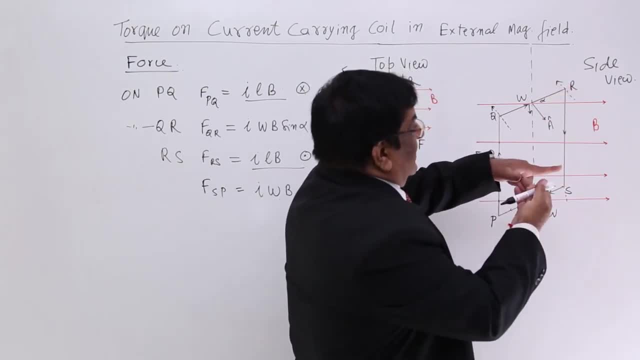 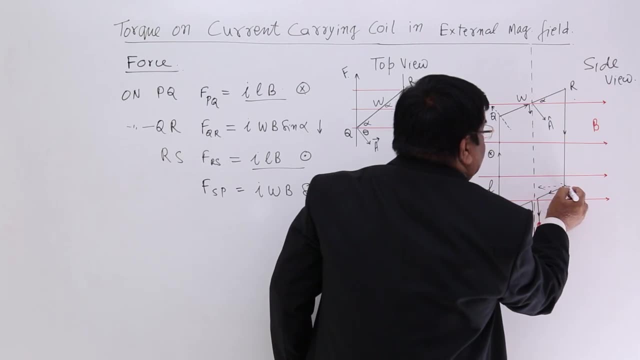 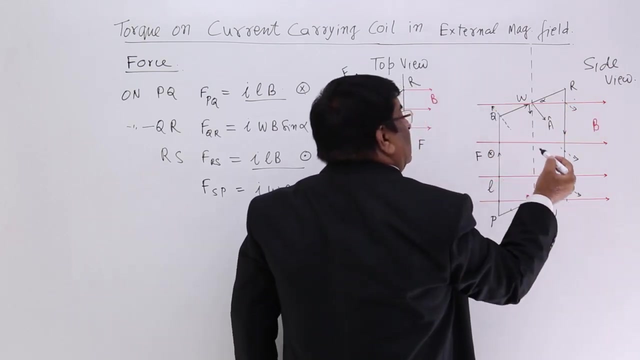 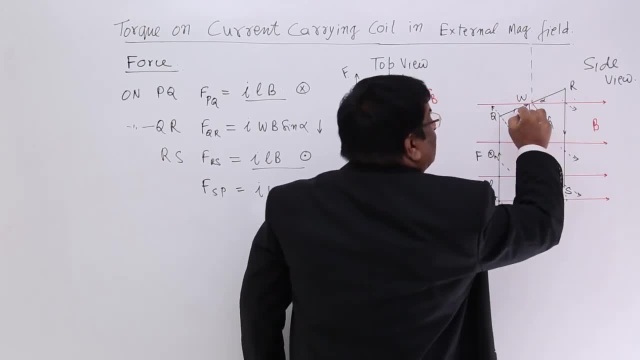 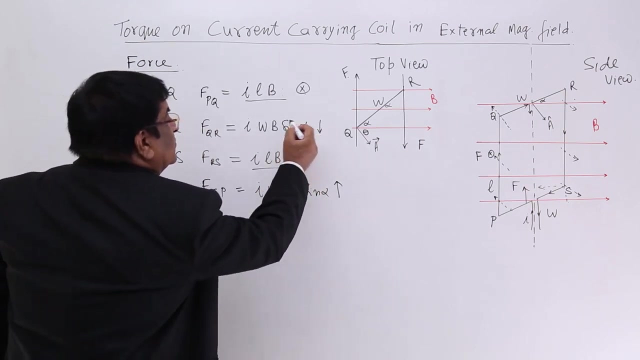 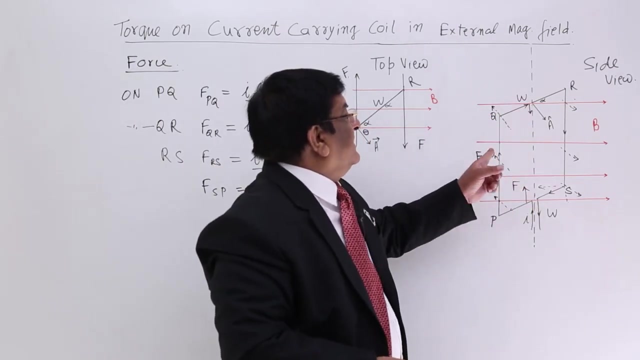 it is going in On this conductor, coming down on this conductor. the force is up, This is force. Okay, now these forces are equal and opposite. cancel out and these 2 forces. This is down, this is up, This is down, this is up cancel. This is in, this is out, cancel. 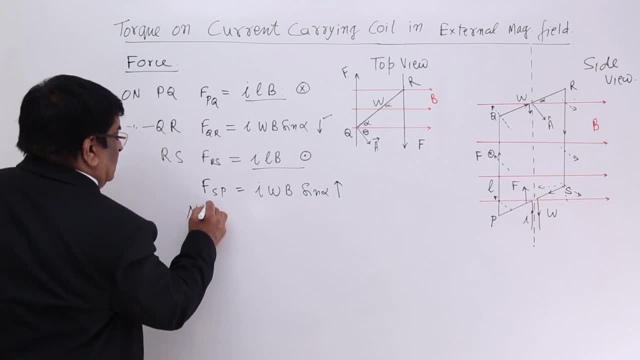 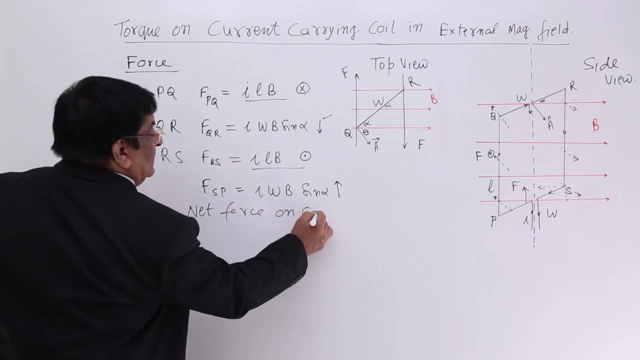 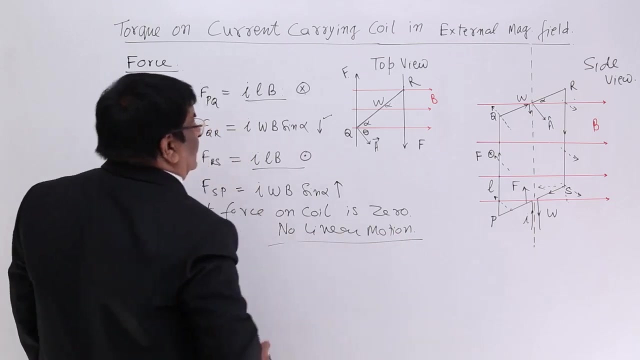 So what is the net force on it? Net force on coil is 0.. Okay, so net force on coil is 0.. No linear, No linear, No linear motion. So remember answer for this question: what is net force on a current? 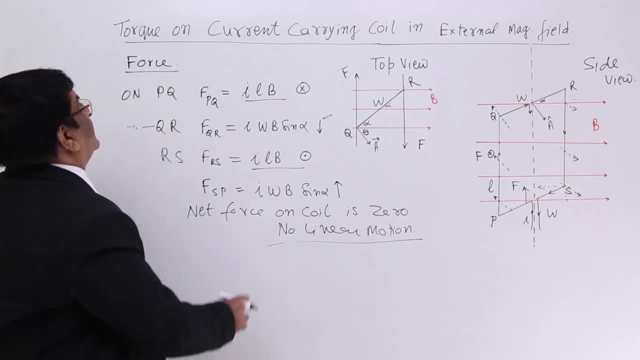 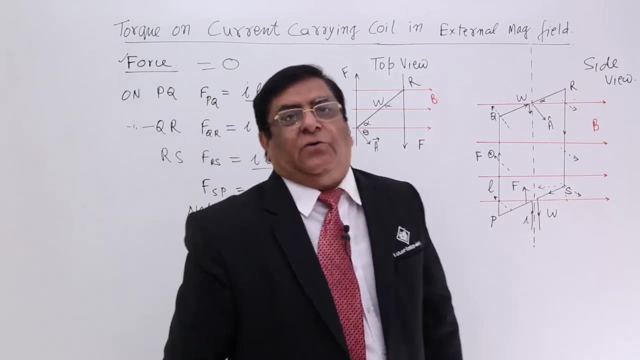 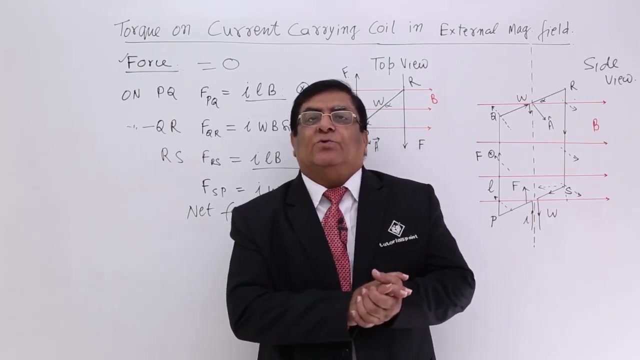 carrying coil in external magnetic field. Mind the word. what is the net force? So answer is: net force is 0.. Okay now if net force is 0, is the net torque also 0?? Answer is no. Who creates the torque? A couple of force creates the torque. And who is the force? 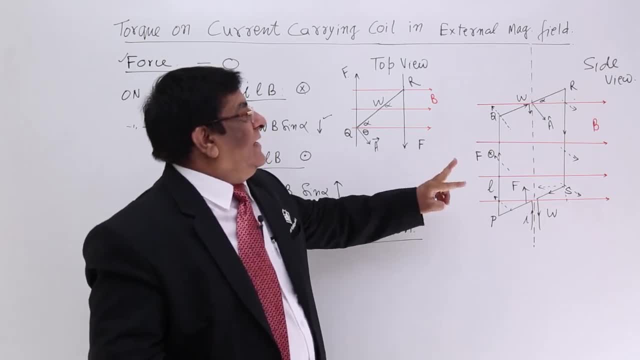 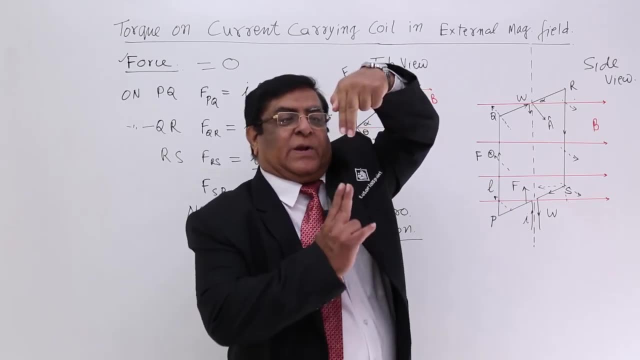 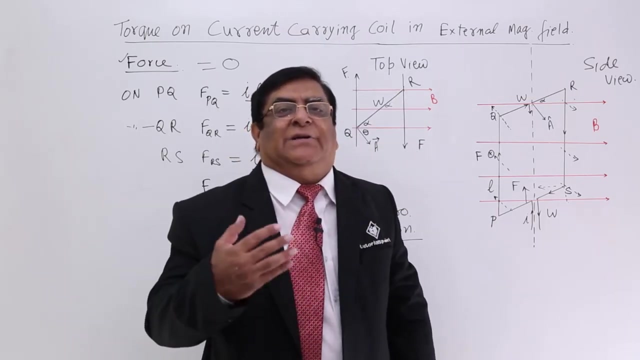 The torque creates the torque And who is couple of force here? Answer these 2.. Do they make a couple? This is working down, this is working up. They are linear and cancel out each other. They do not make a couple because, for the couple, what are our conditions? 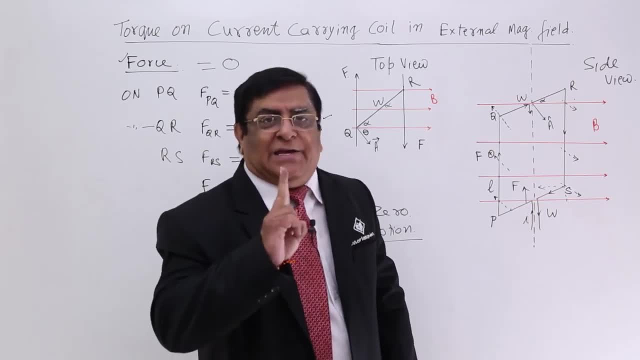 Our conditions are: the 2 forces should be anti-parallel to each other and acting at different points of a single body, Once again anti-parallel to each other. So this is the net force on a current carrying coil in external magnetic field. So this is the net force on 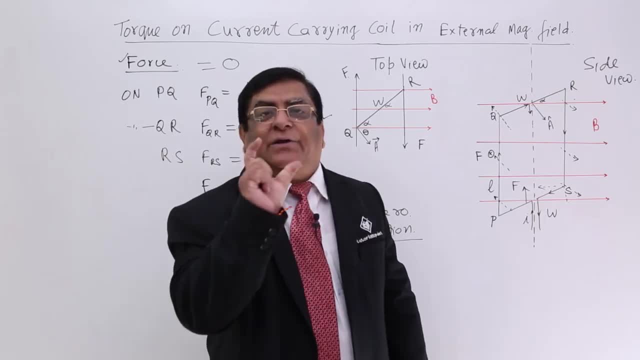 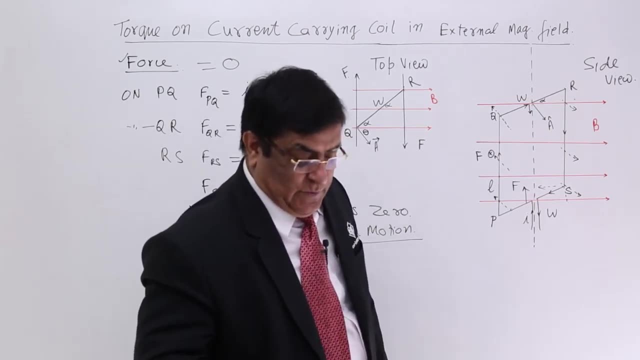 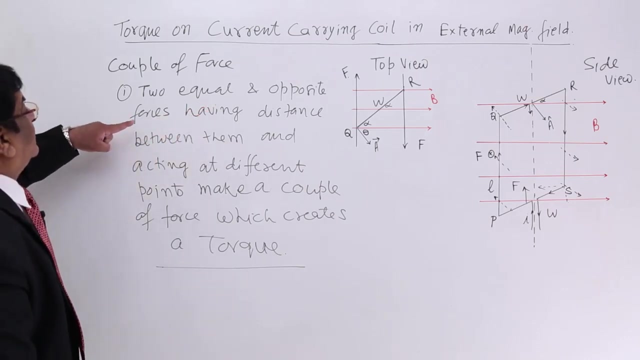 the current carrying coil in external magnetic field. Their magnitude should be equal and opposite: Okay, Their magnitude should be equal and opposite: Okay. So these 3 conditions we write here for a couple: 2 equal and opposite forces having distance between them and acting. 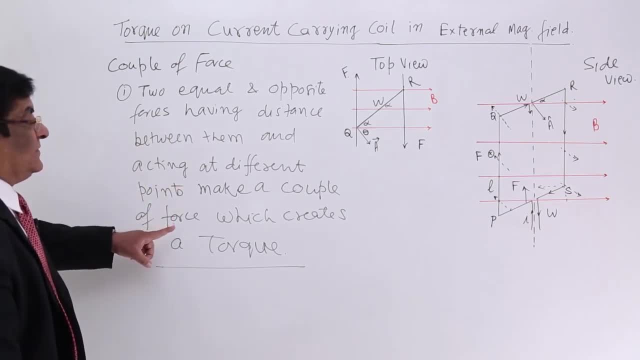 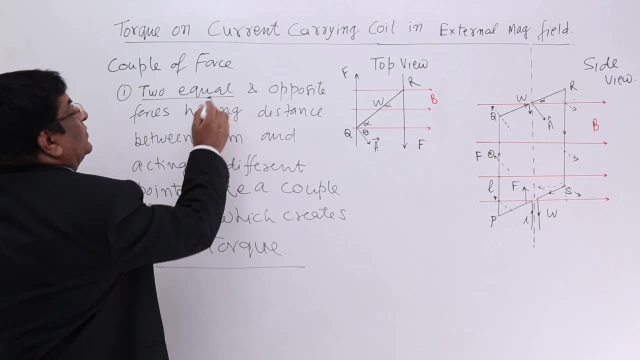 at different points make a couple of force which creates a torque. These are the conditions. Now that I have shown you, I hope you enjoyed the video. Thanks for watching. Bye for now. Now, in this coil, there are two equal and opposite forces. one is this and one is this: 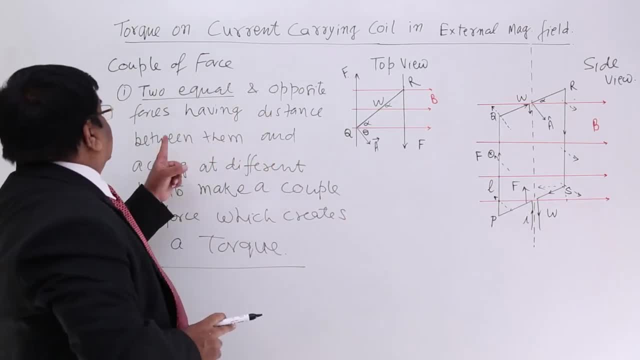 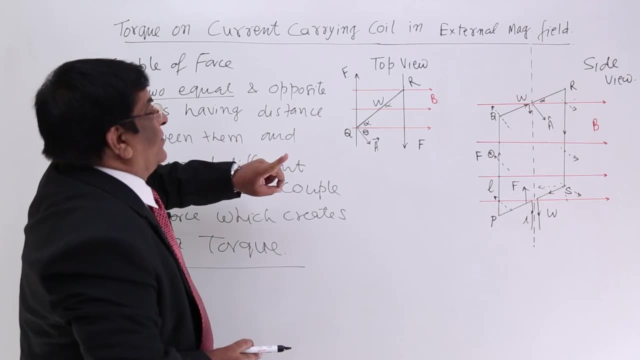 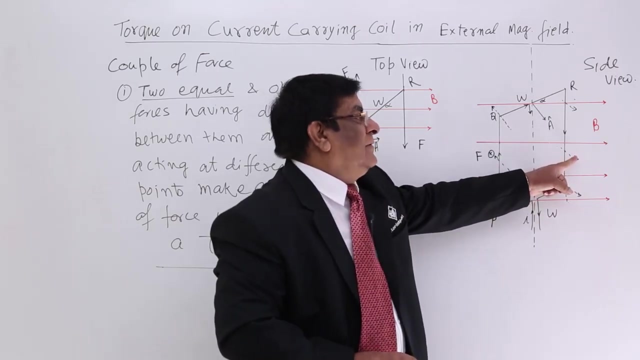 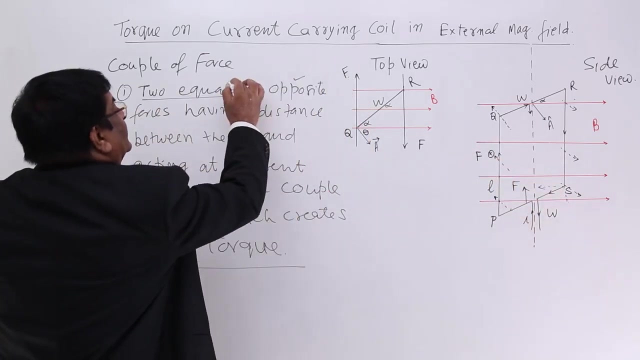 Let us take these two forces having distance between them, two equal and opposite. equal in magnitude. Only these two are equal in magnitude and these two equal are in magnitude. So we will check: equal, yes, opposite, yes, equal, opposite. Distance between them. there is a distance between them. 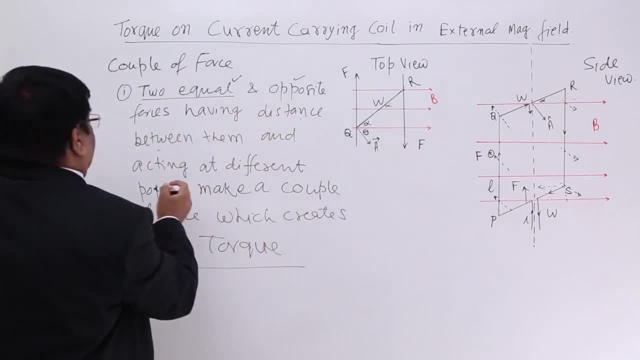 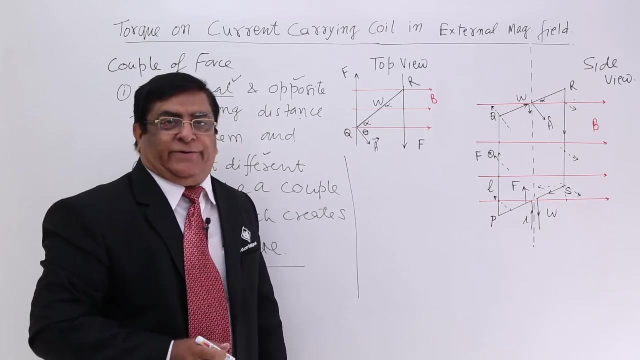 This force, this force? answer: yes, there is difference between them. Acting at different points- yes, there are different points- make a couple of force. So this will make a couple of force And this couple of force will create a torque. 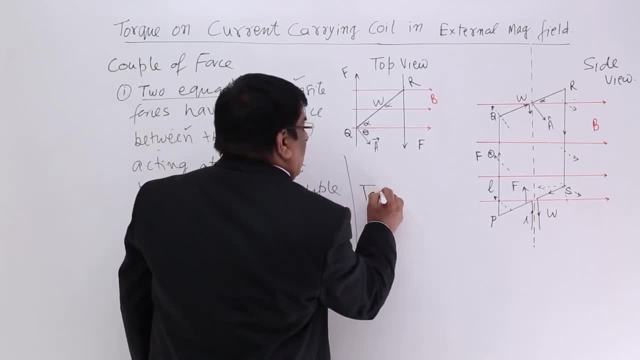 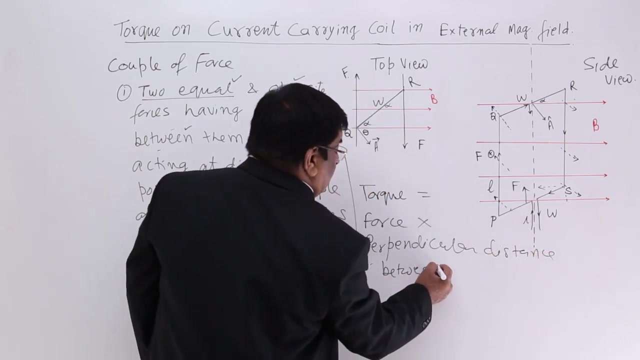 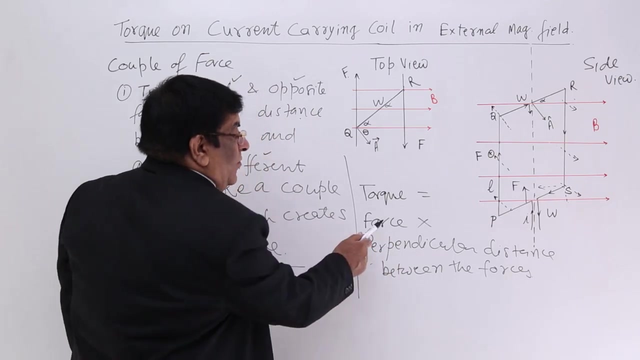 What is the torque created by a couple of force? We have the formula in mechanics and that says force into perpendicular distance between the forces. So I will write here: torque is equal to force multiplied by perpendicular distance between the forces. This is formula for torque: multiplication of these two things. 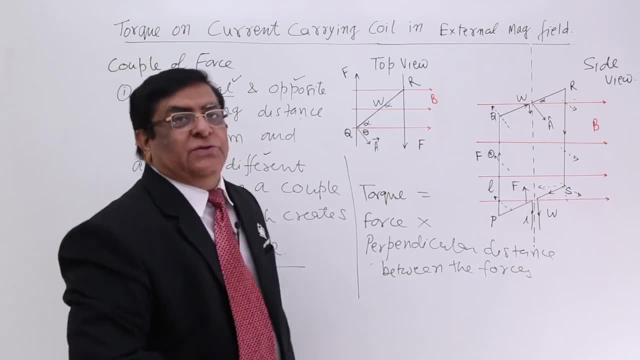 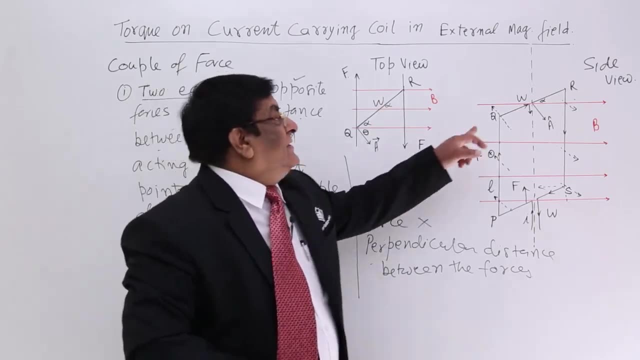 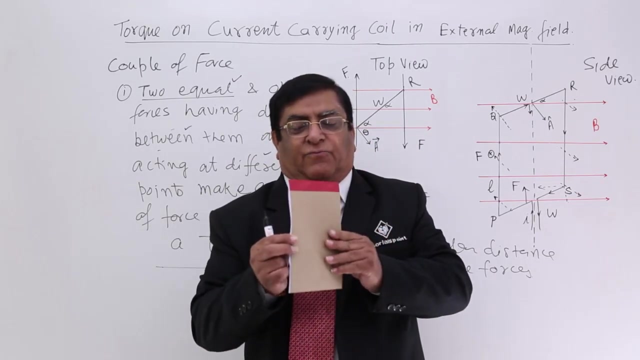 Now I want to find out what is the magnitude of this torque. So I must have two forces indicated in a vector diagram. I make it here This: if you see it from the top, if this is the coil and it has rotated somewhat and I 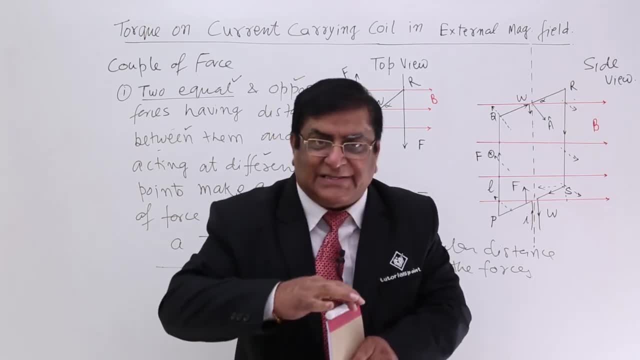 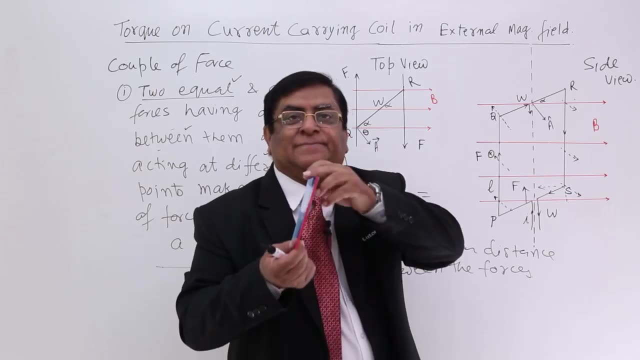 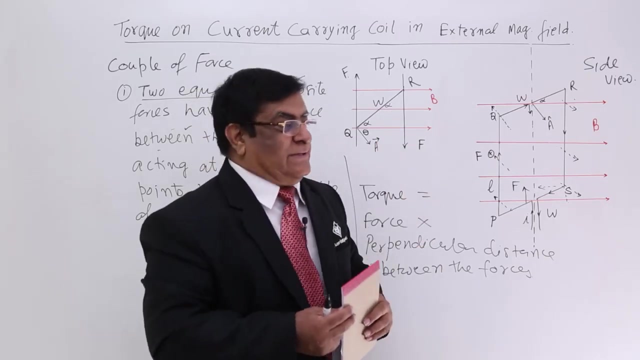 see it from the top. What do I see? Only this W line, which is QR line, and when you see it from the top, it will be like this: So you see this one line, that is what I have shown here- QR. and what are the forces? 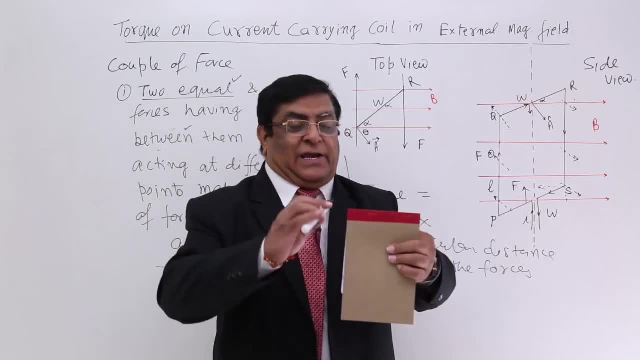 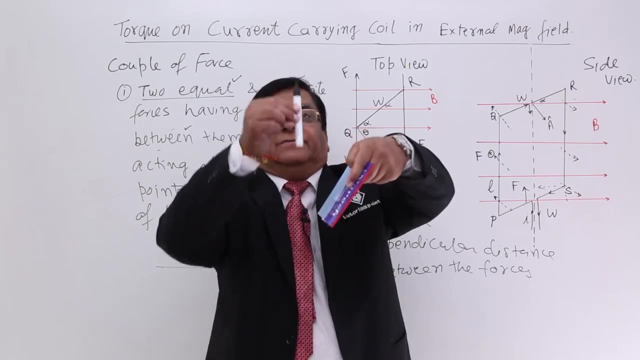 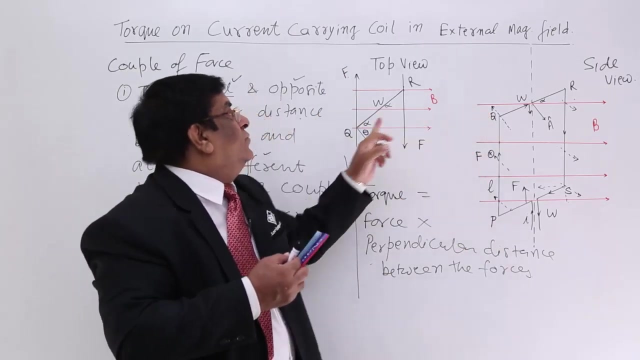 On this side, the force is acting inside this way and when you see it from the top, it will appear like this force working here. this And this I have shown here, This is the force acting on this PQ and here the force is acting on this. the force is. 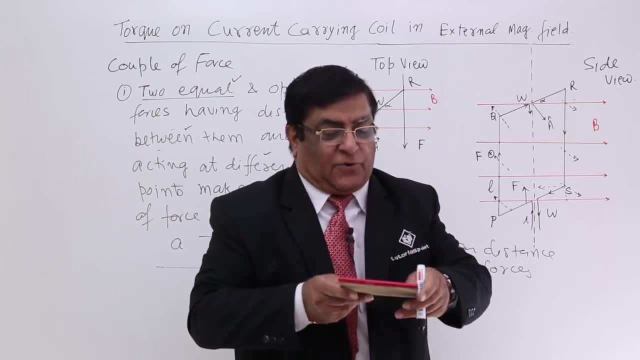 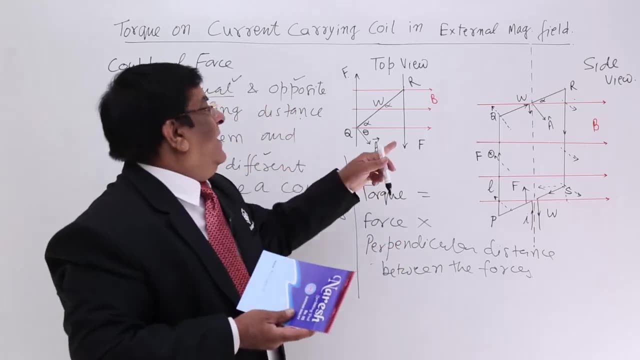 acting this way And if you see it from the top, this way or this way, the force is acting this way. So this I have shown here. So this is the top view. this helps us to calculate. Now, only coming to the top view, 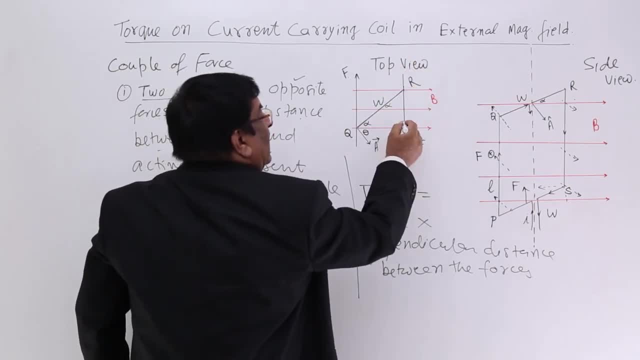 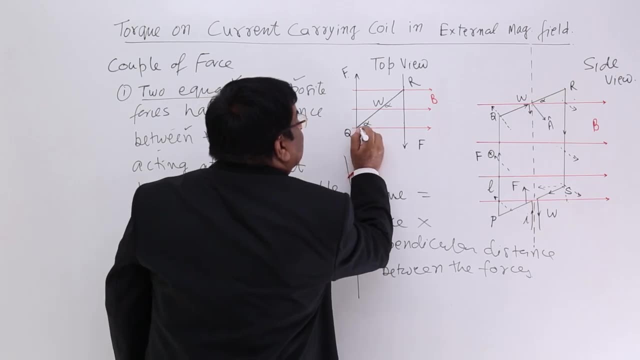 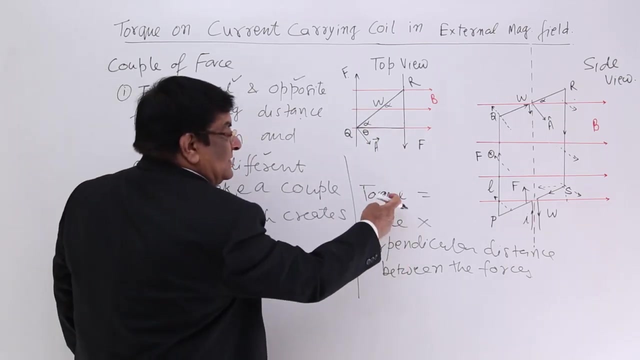 The force on the column is acting on this PQ. So this I have shown here. So this is the top view. The force on the column is acting on this PQ and here PQ is on this curls PQ. The force on the column is acting on this PQ. 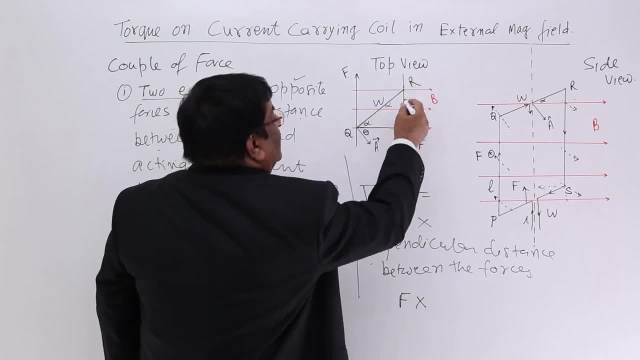 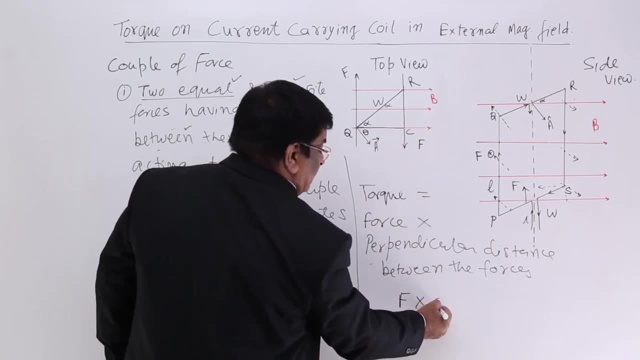 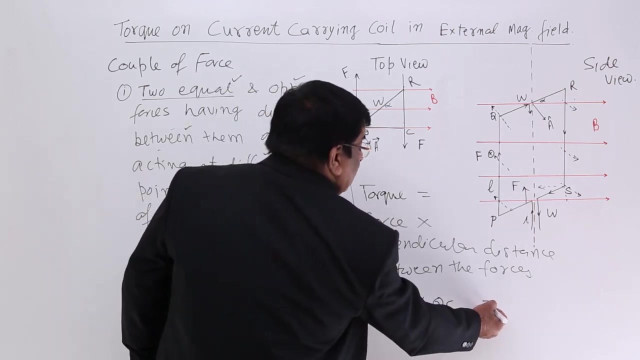 And this will be acting on this angle point. So this will be Qc, the perpendicular distance. Qc, force into Qc. this is the torque. Now we will put value here and this is the important thing. you should understand: force. 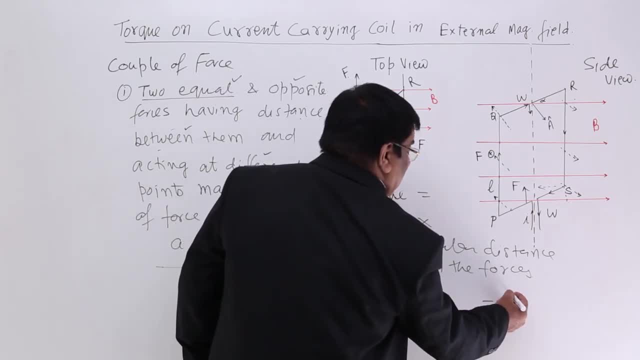 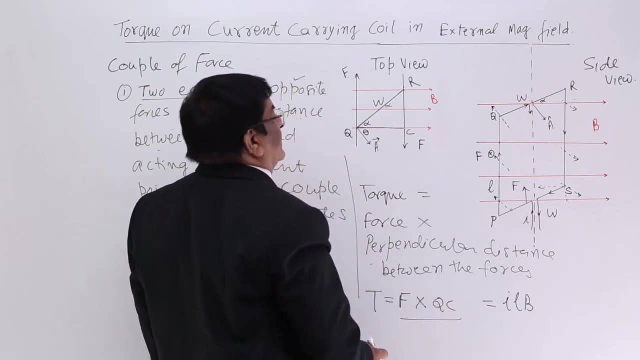 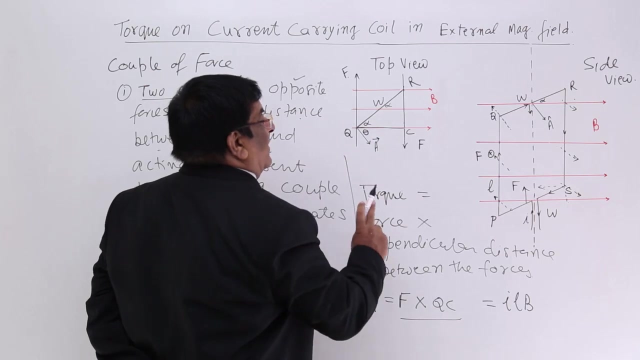 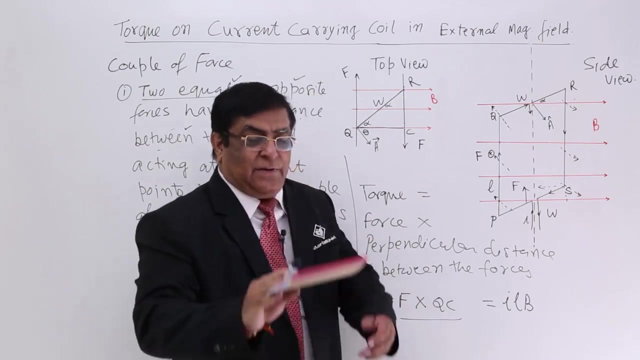 on each conductor. we have already calculated. this is I lb. this is the force calculated. Qc: how much is Qc For Qc calculation? this Qc, this can be calculated with respect to two angles. What is this? If this is, I am telling you: this is the coil. where is area vector of the coil? 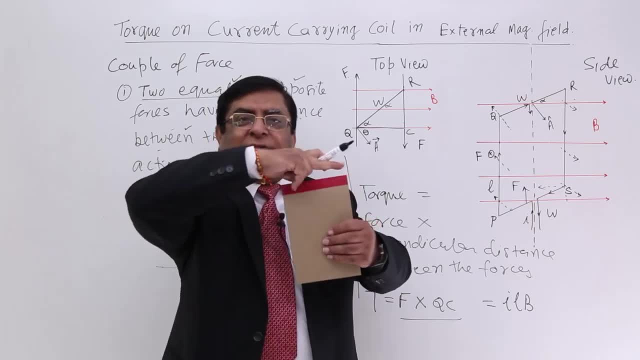 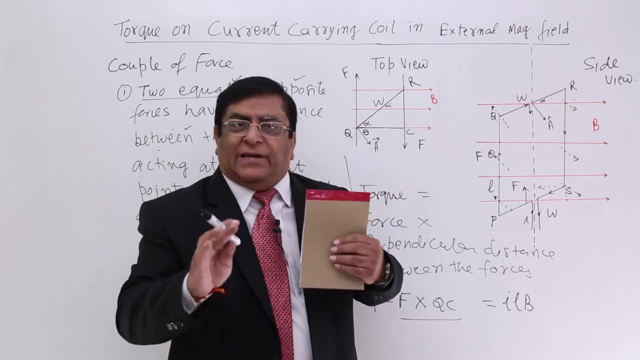 It has got a length in this direction, it has got a width in this direction. then what this? where is area? This is area. what is direction of the area? So we have done it many times: direction of the area is this. 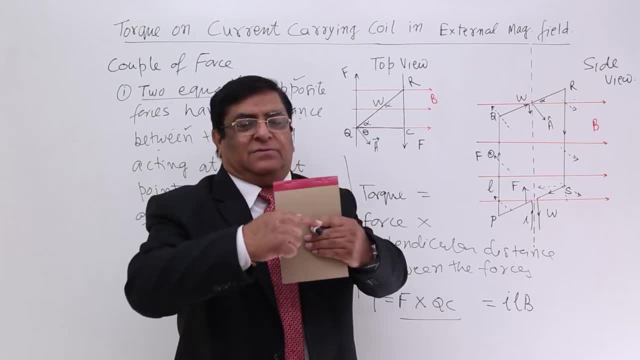 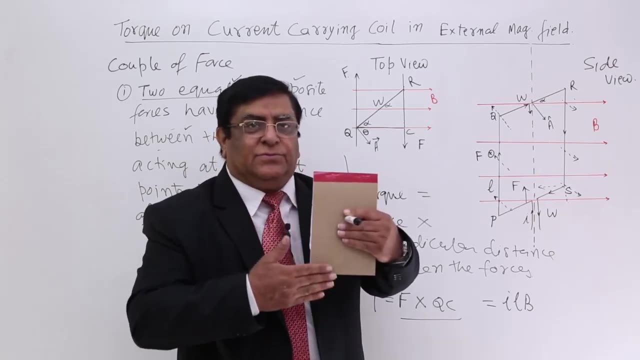 So if this is x, this is y, this is z, if this is x, this is y, this is z. whatever it is, But a perpendicular to surface is known as area vector. this is area vector, so how should? 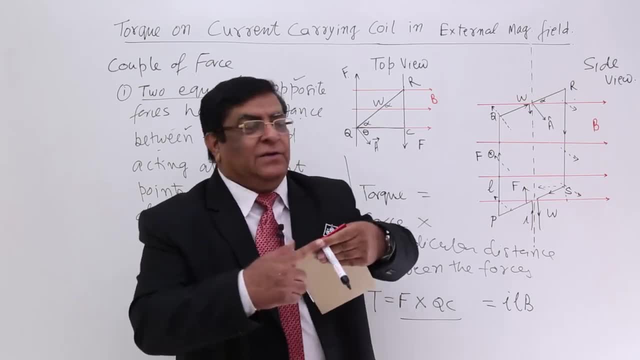 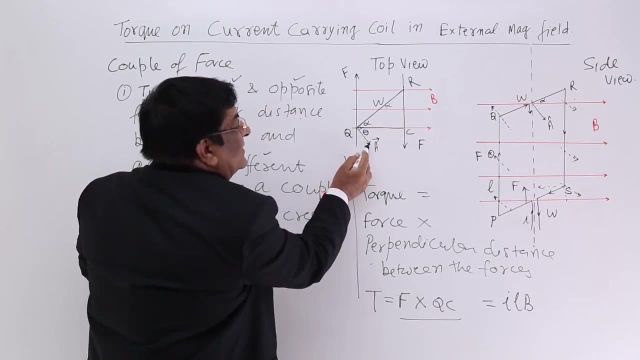 I draw it. I should draw it normal to this line, so I have drawn it normal to this line. this is 90 degree, So what is this direction representing? This direction is 90 degree, So what is this direction representing? 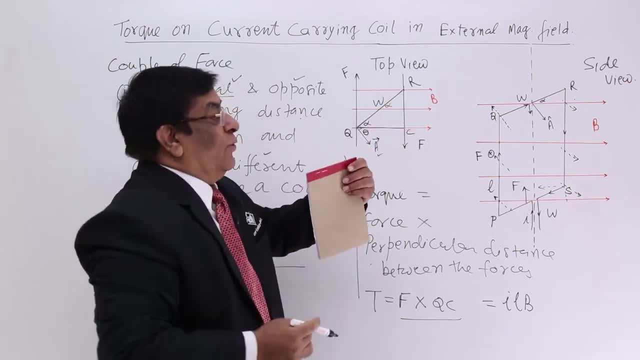 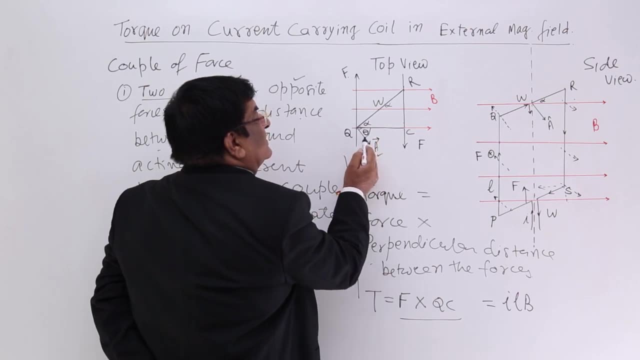 This direction is 90 degree. This direction is representing area vector of the whole coil. Now, this area vector, this is magnetic field. the angle between the two is theta and this is the important angle for us, because this is angle between area vector and magnetic. 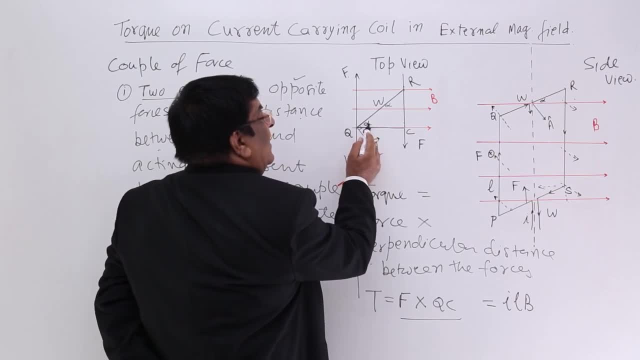 field. If this is theta, this is alpha. what is alpha? Alpha is 90 minus theta. If this is alpha, how much is this angle? This is 90,. this is 90 minus alpha, But 90 minus alpha is theta. 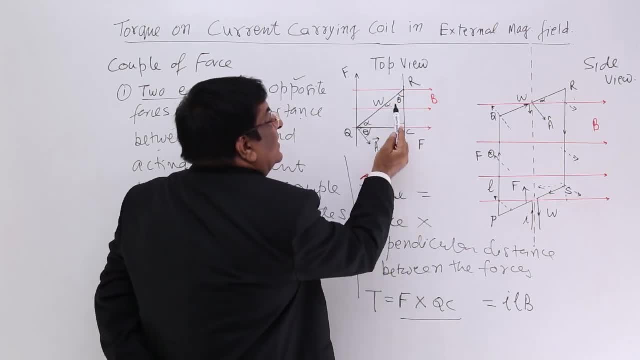 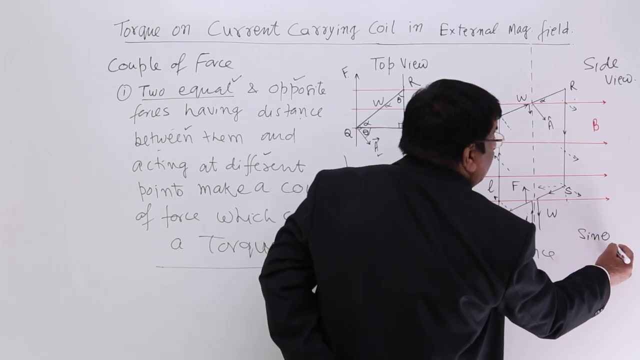 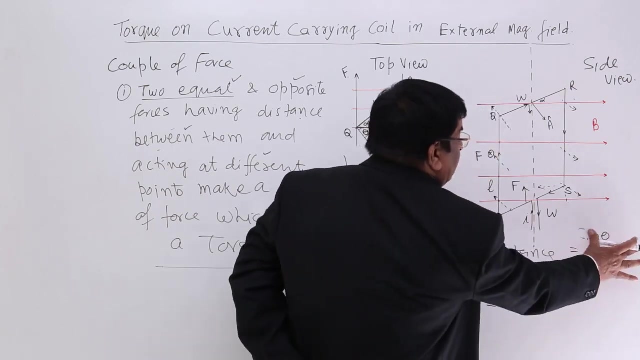 theta. So I can say: this is theta. Now, if this angle is theta, what is sin theta equal to? So sin theta is equal to perpendicular Q c upon Q r, So I will mention it here: sin theta is equal to Q c upon Q r. So what is Q c equal to Sin? What is Q c equal to Q? 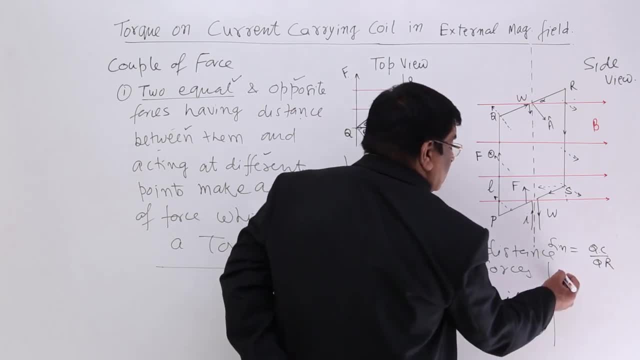 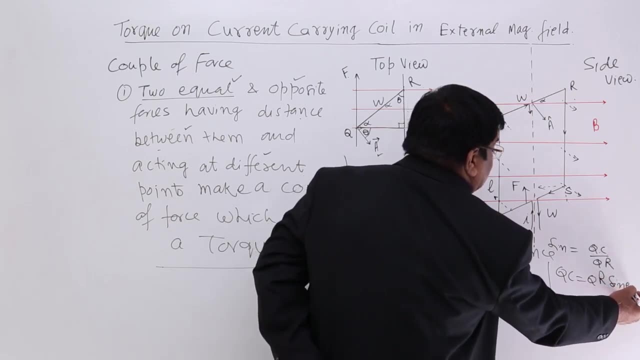 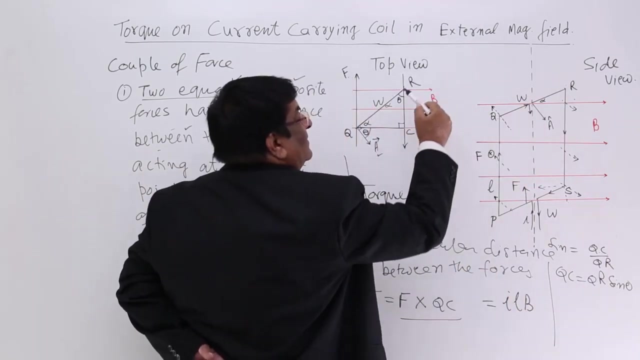 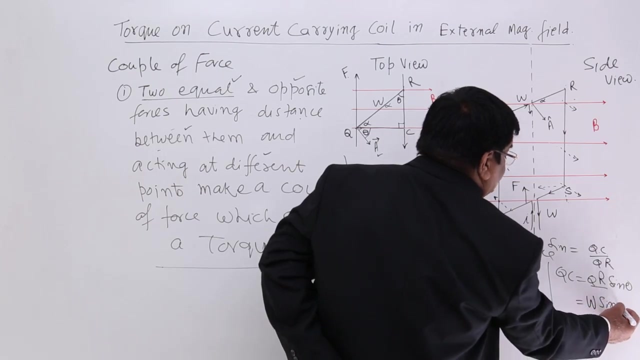 r into sin theta. So Q c is equal to Q r into sin theta. Now, what is this? Q r equal to This is equal to width of the coil. So this we can very well write W into sin theta. This. 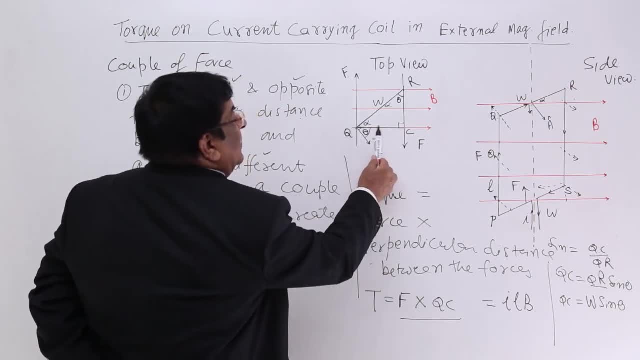 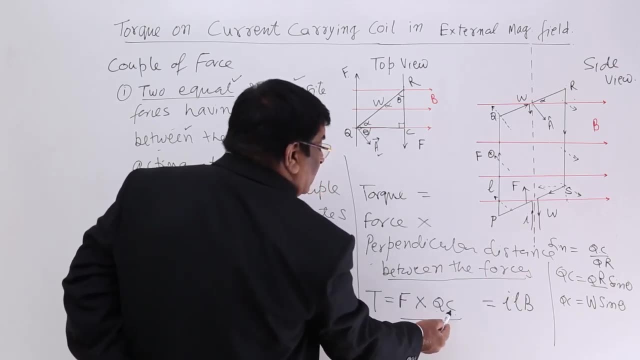 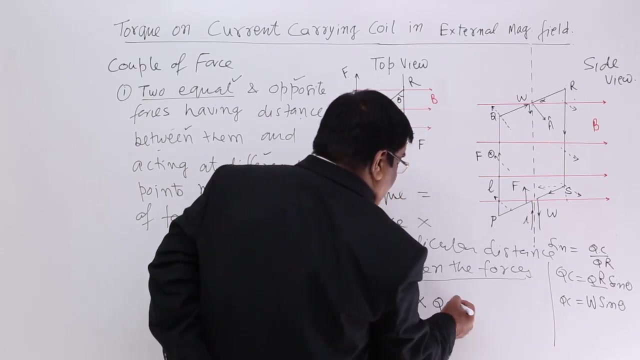 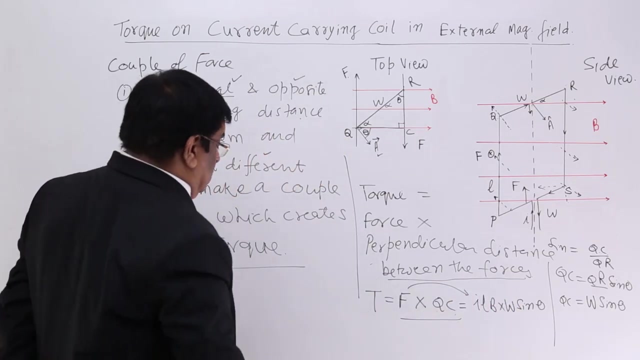 is what Q c and what is Q c. Q c is perpendicular distance between the two forces which we need here, between the forces Q c. So this force is equal to I l b and force is equal to I l b multiplied by Q c. we will write as: W sin theta And this gives you. this gives you. 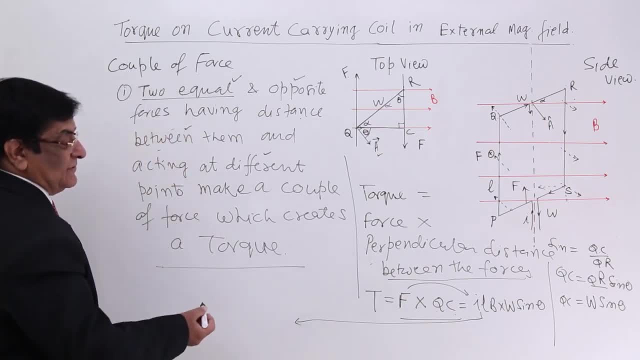 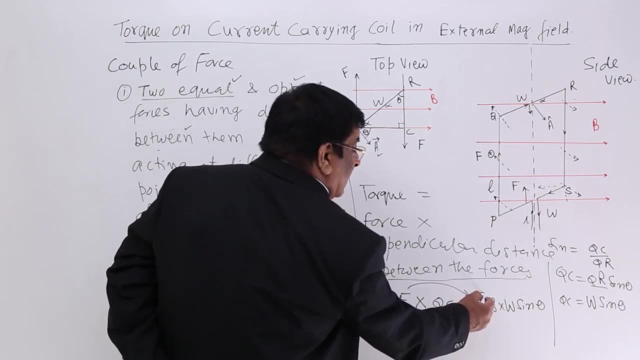 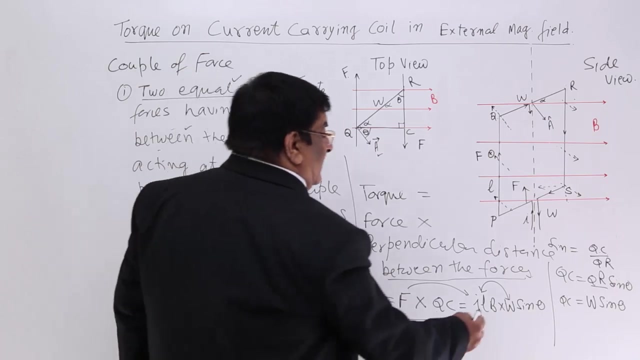 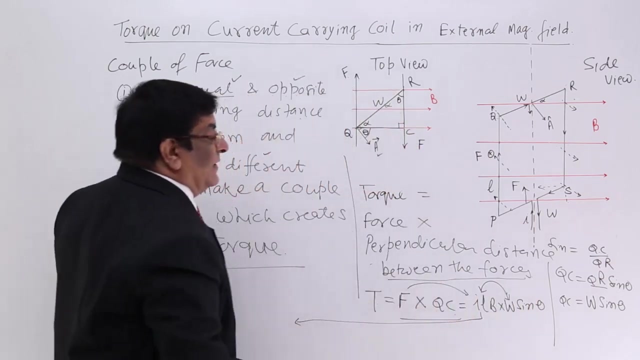 again a formula which is Torque is equal. to see here length multiplied by width, Length into width, into sin theta. What is this formula for? Or let us forget sin theta First. we make only length into width, Length into width, for any coil is its area. So this we can write as torque is equal. 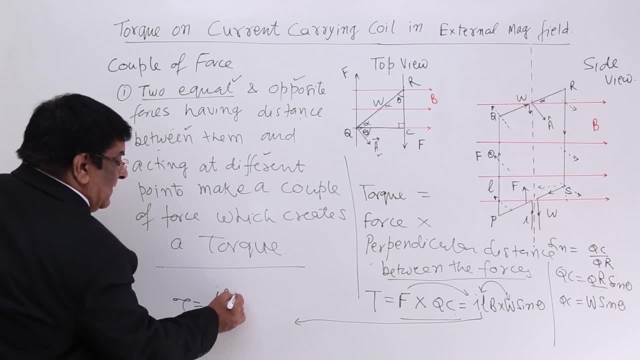 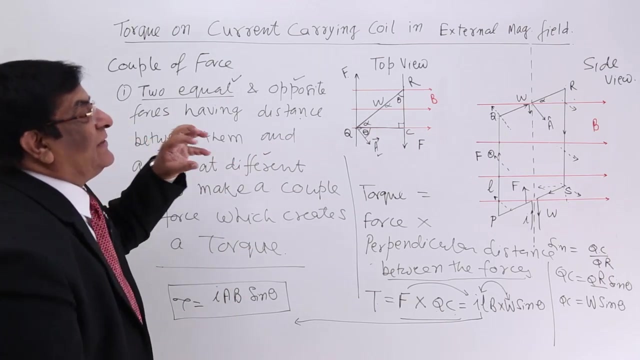 to I, area l, area b, sin theta. Well, It has come. what is I Current flowing in the coil? what is a Area of the coil? what is b Strength of the external magnetic field? So this is the torque created. Now, if we have, 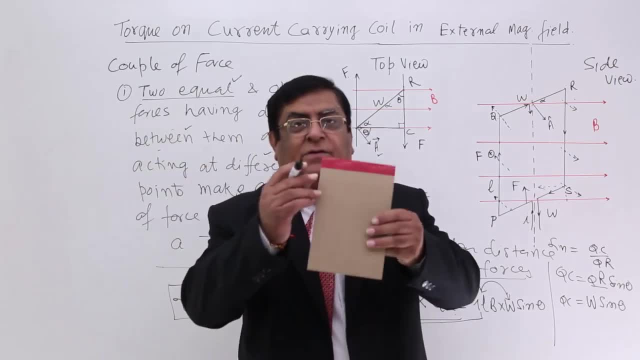 number of turns in the coil. here we have 1, 2, 3, 4, n turnsuttic So we can write CR through. the walk of the coil will be the flow. We can write as Q 3 into N. Now it has come one Q c into Q c. We can write A into W, sin theta We are able to do another. 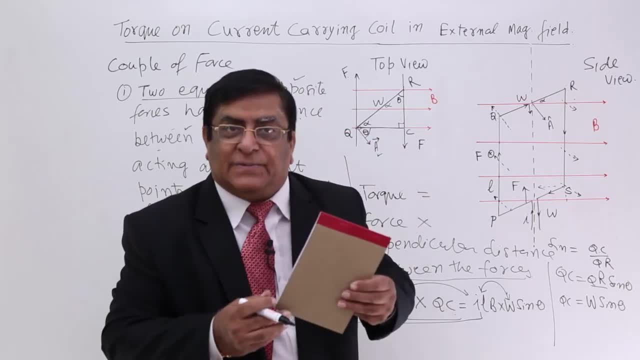 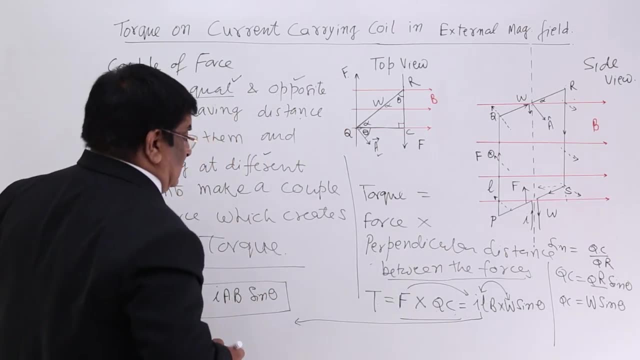 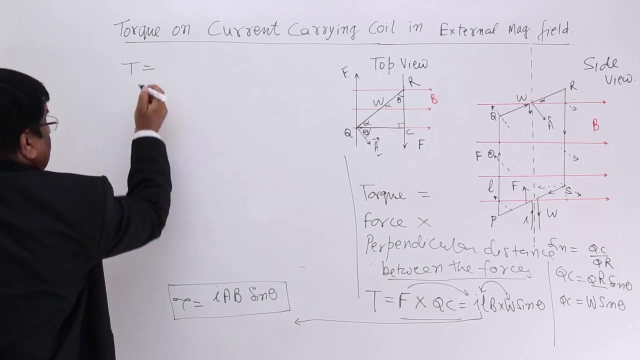 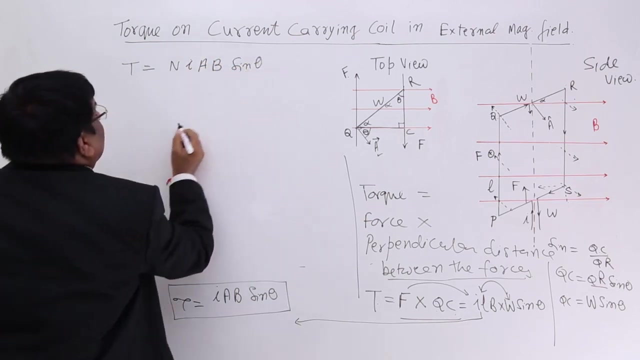 Sr delta, We have to write cool here which is x, stays e, So this we can write as 1 H, So this n turns. so there will be n torques which will be added together. so total torque will be for n turns, so torque for n turns. so torque for n turns will be n. i, a, b, sin theta now. 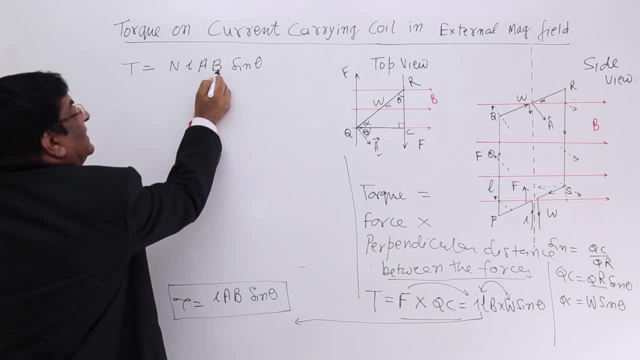 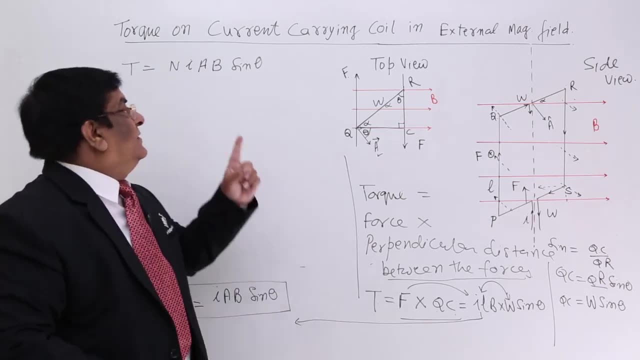 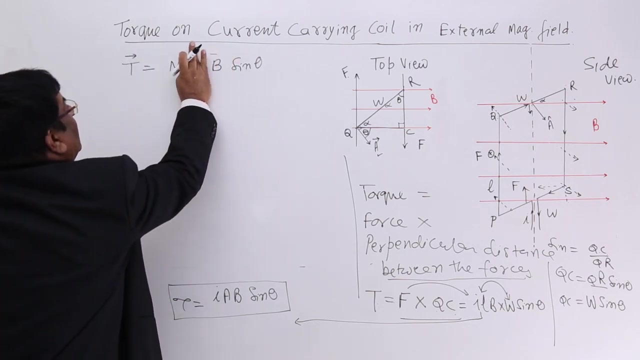 here theta is angle between vector a and vector b. and what is cross product of vector a and vector b? cross product a cross b is equal to a b sin theta. so this torque is a cross product of area and magnetic field. so I will write it here: torque in vector form n number. 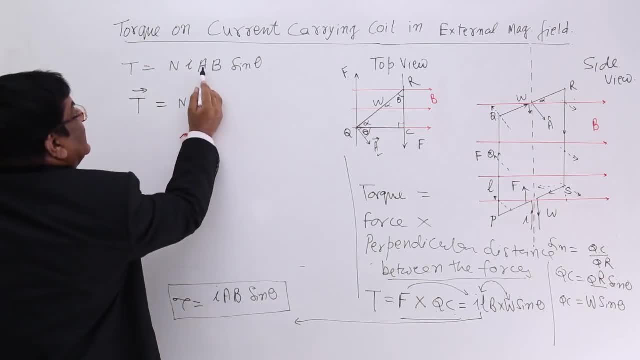 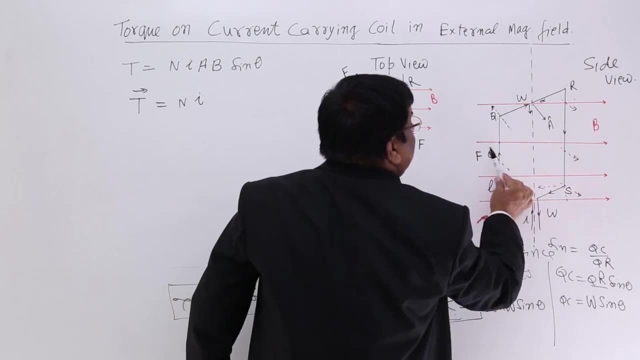 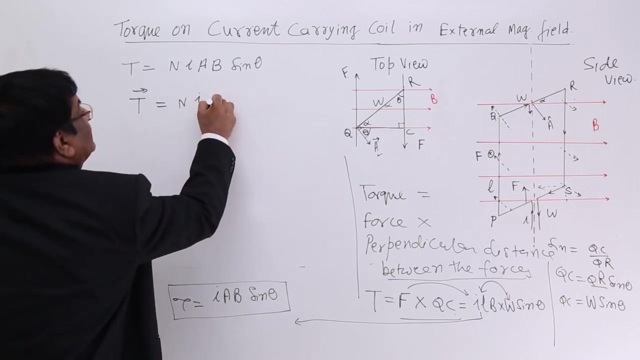 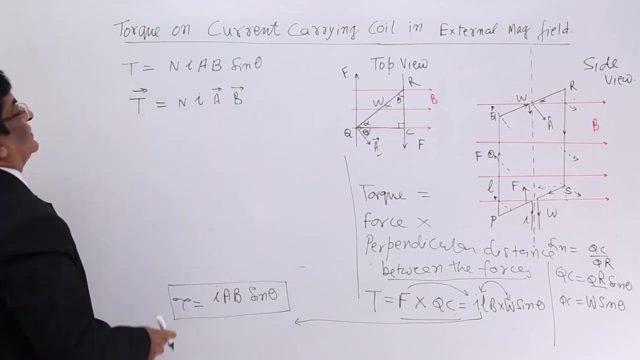 of turns. scalar quantity i is a scalar quantity. it is an multiplication of two vector quantity: this area, area vector, and this is magnetic field. So ni, this is area vector and this is magnetic field. So this gives us the torque, niab. and when we have to write the magnitude, we will 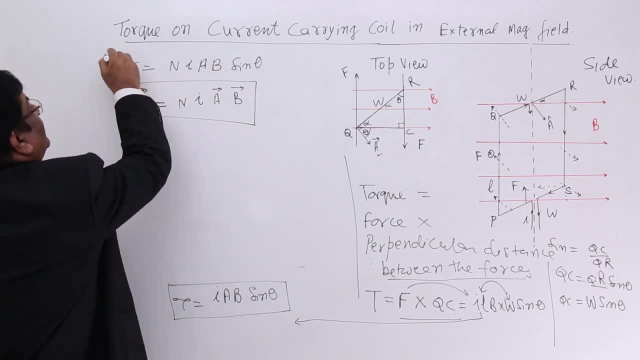 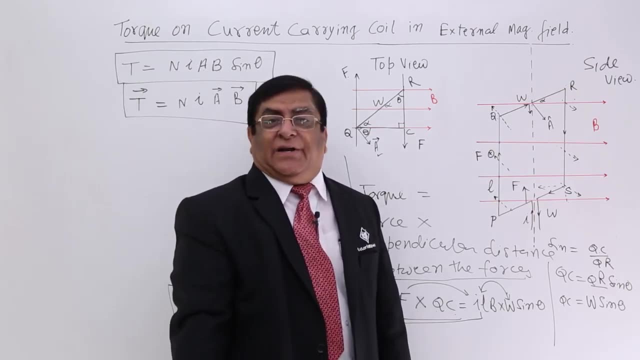 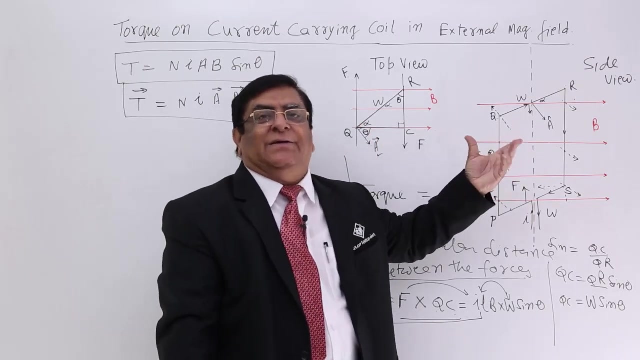 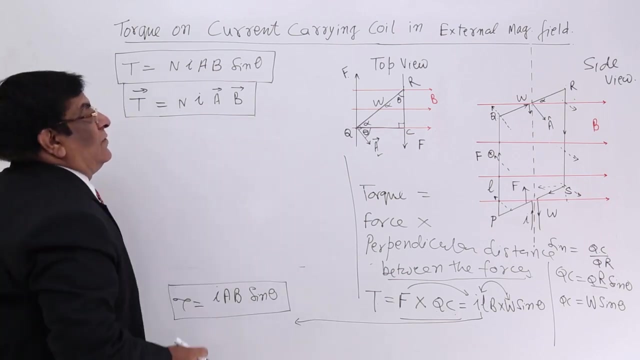 write it: niab sin theta. Please remember both the formulas. these are very much required whenever we study about motors, whenever you study about generators and anything which is rotating in the magnetic field, whether it is generator or motor or anything- you will need this formula. So this is the formula for torque created. So what happens if a current 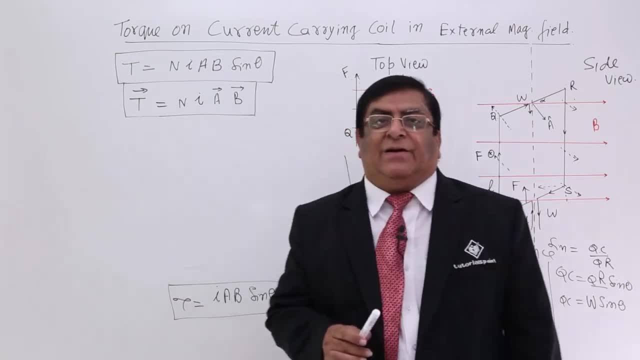 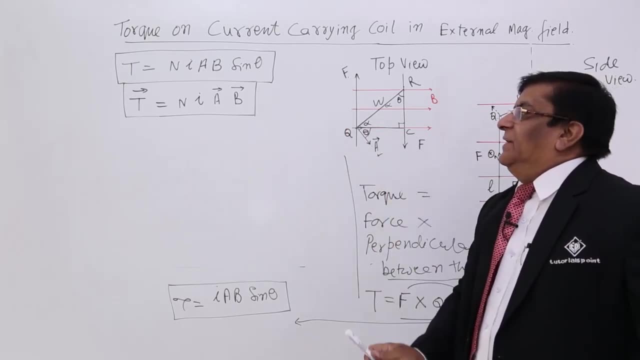 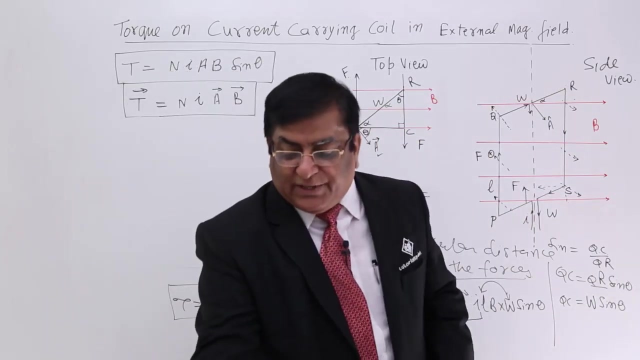 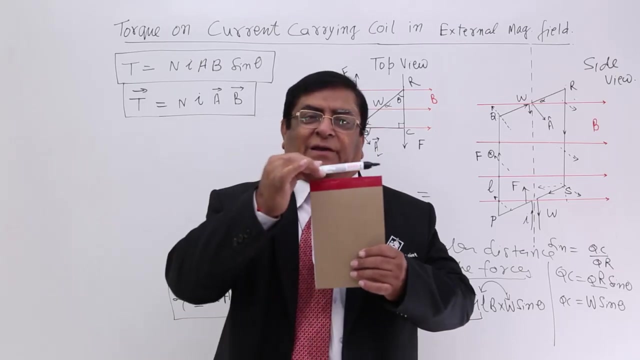 carrying coil is placed in a magnetic field. Answer: it experience a torque. How much is that torque? The torque is niab, sin, theta. When is this torque maximum and when this is minimum? So there is a magnetic field and that magnetic field has this direction. It is not moving. Same magnetic field remains. 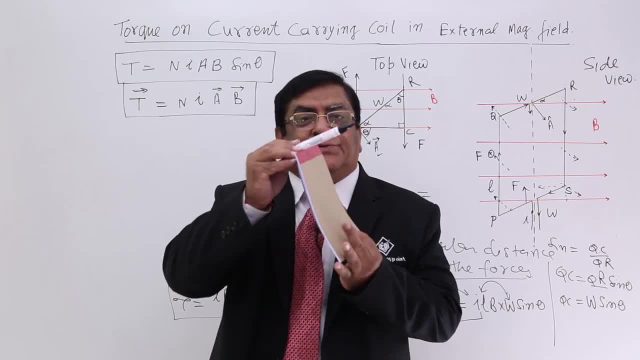 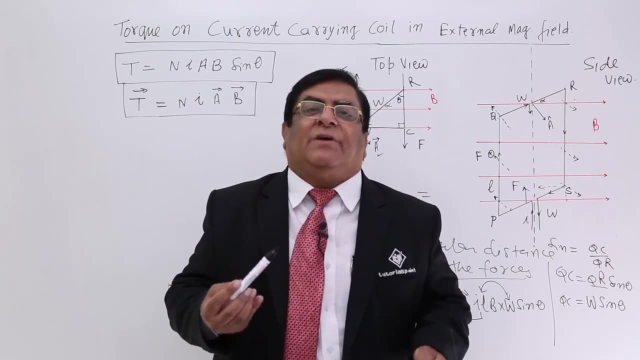 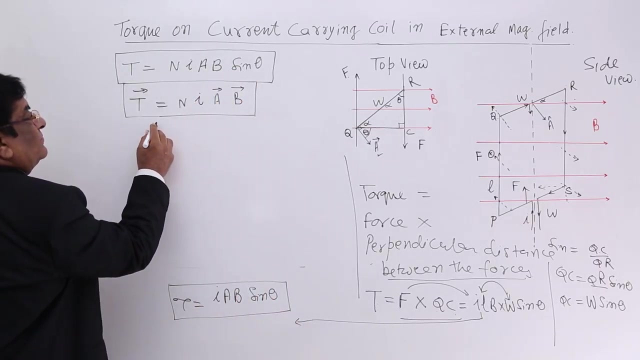 This is moving. Now, when this moves, then at any position, is the torque maximum or is the torque minimum? Answer: yes, We can find it mathematically. How we can find it mathematically That this torque has a magnitude- niab, sin, theta. So torque will be maximum when sin. 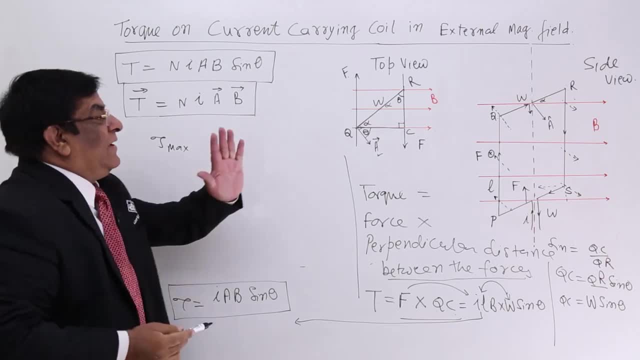 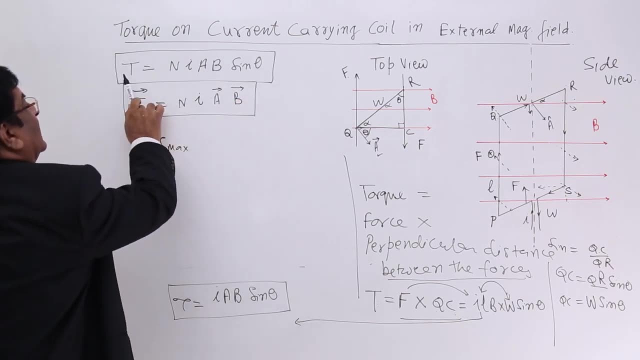 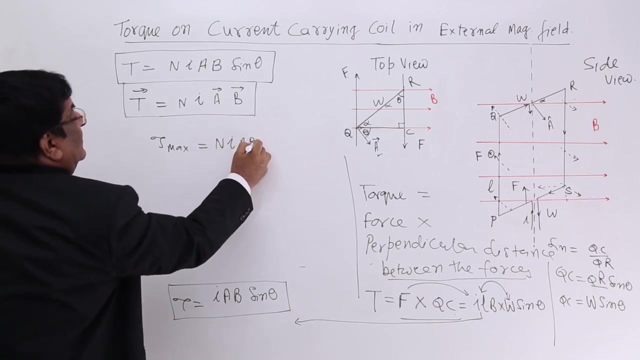 theta is maximum, because this is the variable term. when it rotates, then it is theta which is changing. So based on the sin theta value, we can find out maximum when sin theta is maximum. So this is: how much niab sin theta? Answer: yes, 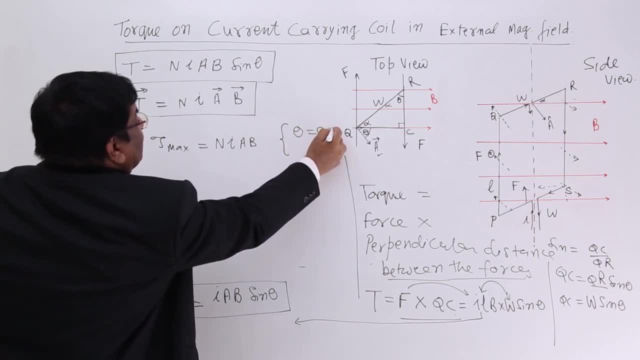 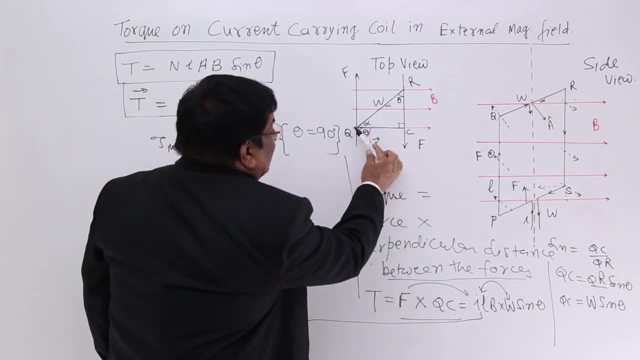 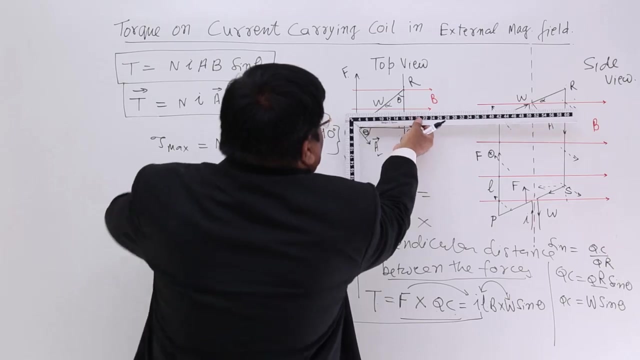 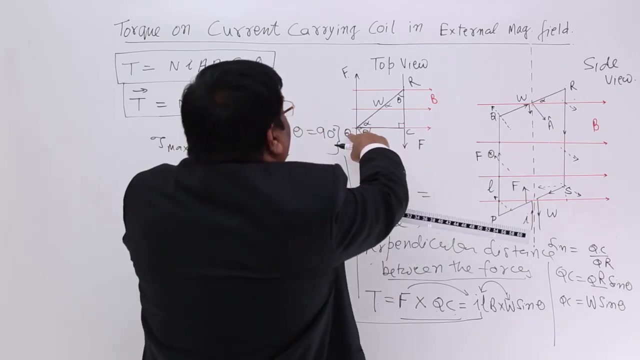 E and here theta is equal to 90 degree. When is theta equal to 90 degree? This theta will be 90 degree. if you see, this is like this and I want to make it this way so that this theta is equal to 90 degree. Where is the coil? This is the coil QR Coils width is: 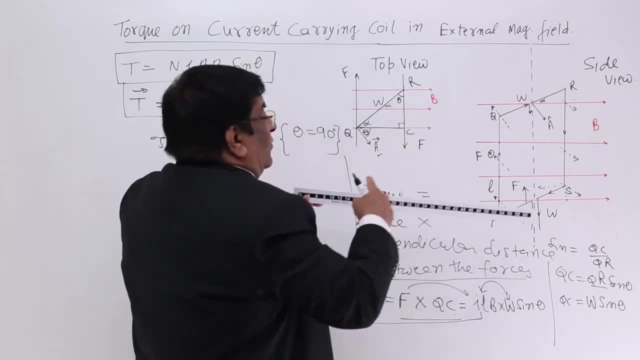 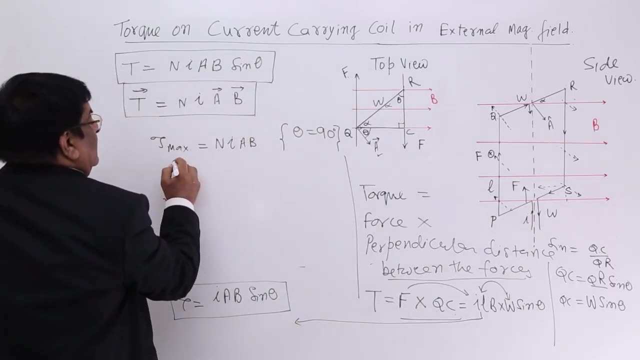 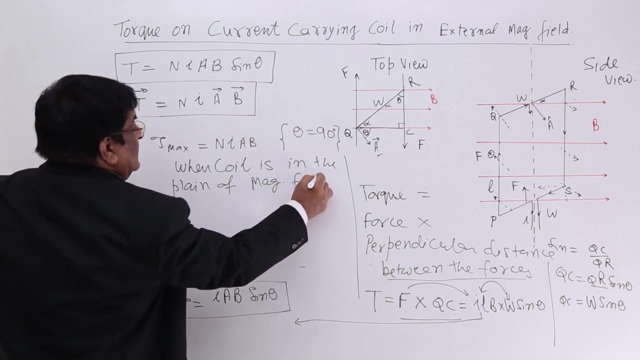 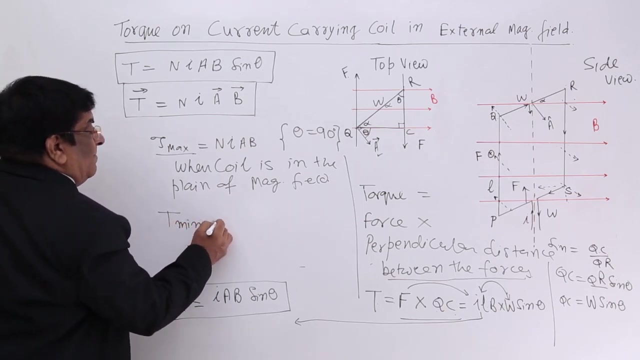 this: Where is the magnetic field? This is the magnetic field. Both are in the same direction. So we declare here: when coil is in the plane of magnetic field, then torque is maximum. and opposite to this, Torque is minimum when theta is equal to 0. and see here: when theta is equal to 0, this: 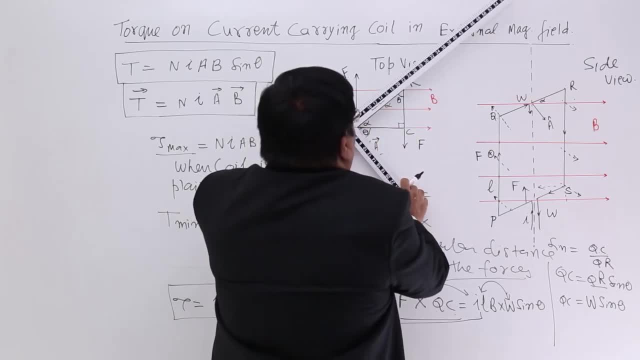 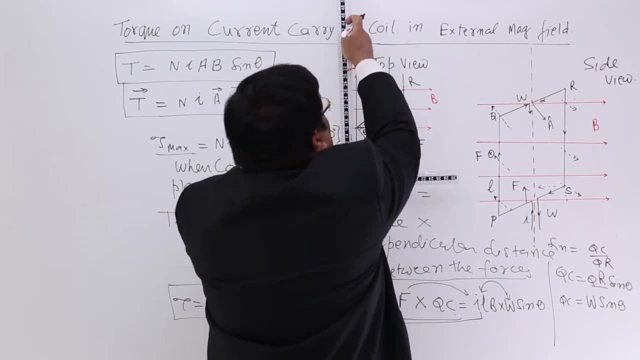 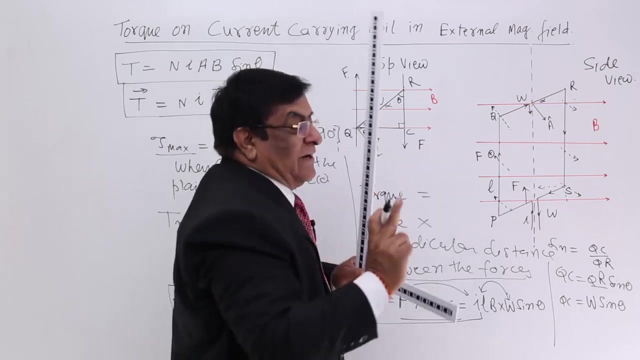 is QR. this is area vector. We want this angle to be made 0, so I make it 0.. How is the coil now? This coil is perpendicular to B. So when coil is perpendicular to B, area vector become parallel to B and theta will be taken as 0. 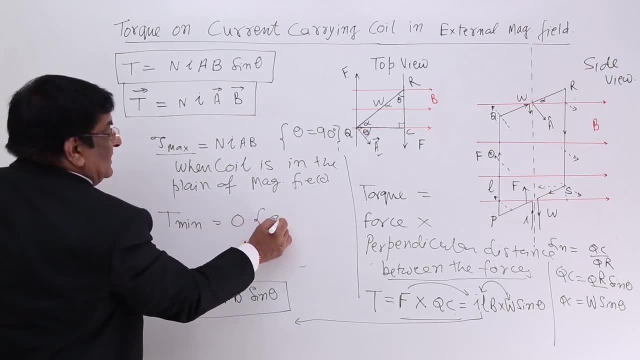 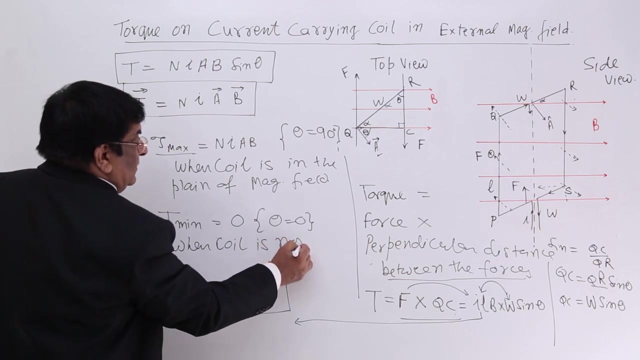 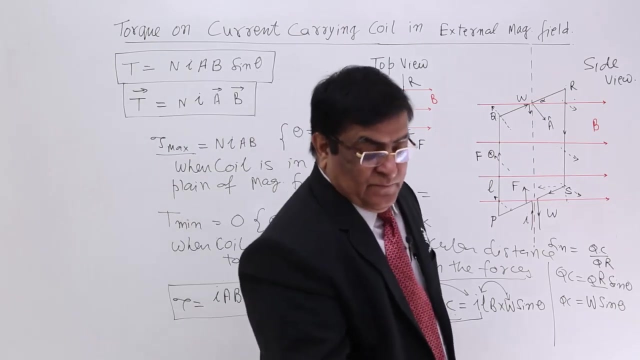 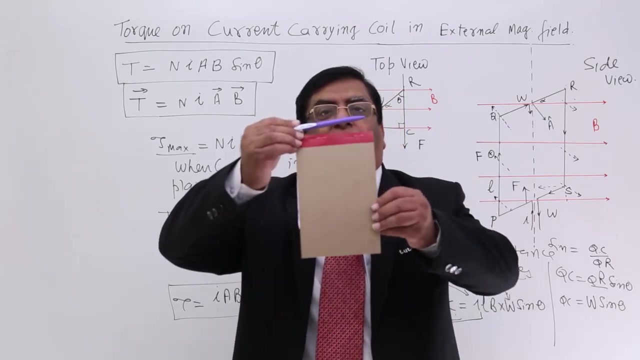 This T will be minimum 0,, theta is equal to 0 and when area vector, theta is equal to 0, when coil is normal to B magnetic field. Okay, So remember, If this is a coil and this is magnetic field, at this situation, how is the torque maximum? 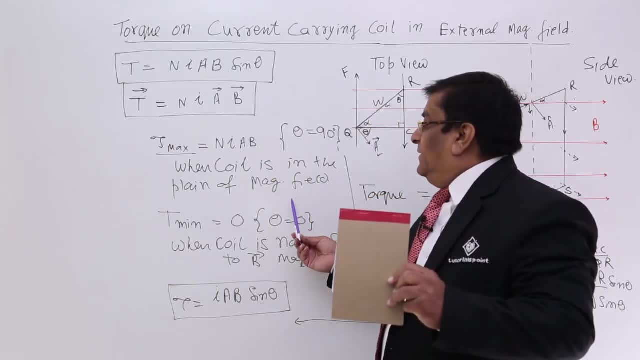 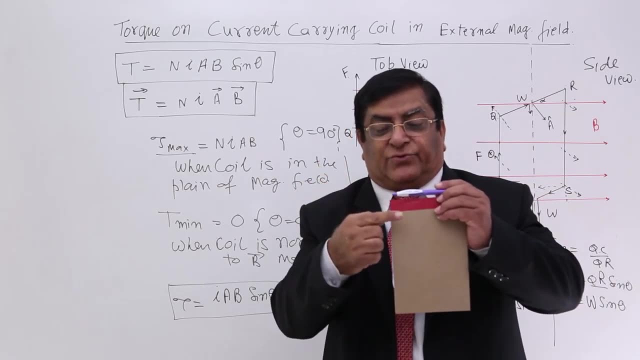 or minimum. Look here and remember: is theta who decides theta? Is it deciding theta? You are very much tempted to say the angle between 2 is 0,. yes, it is 0, but this is not the theta. this is theta. 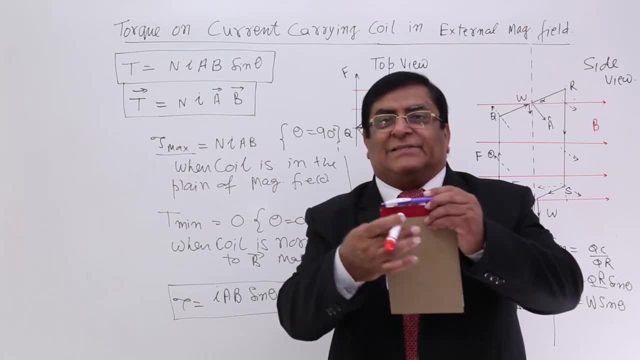 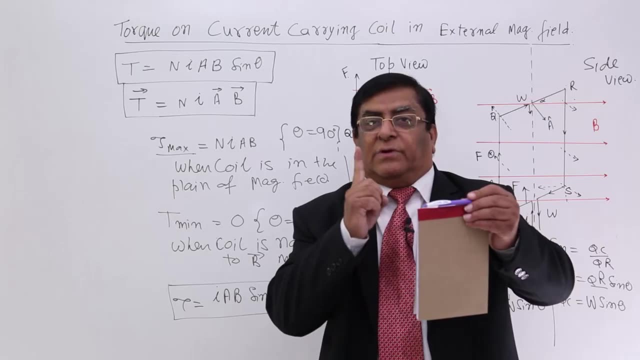 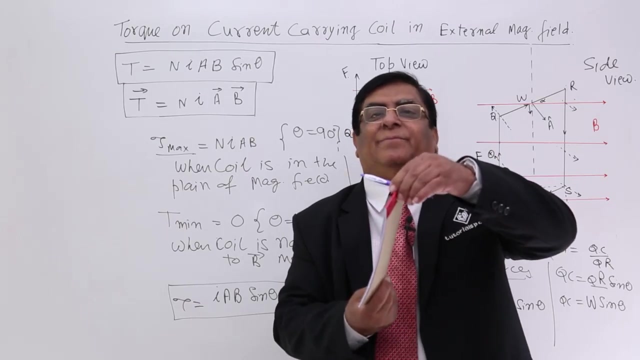 This is area vector, The area vector and this. they are at right angle to each other and at this time this is maximum. So make a thumb rule, remember it: when coil is like this, this is maximum, and when coil is like this, at that time torque is minimum. 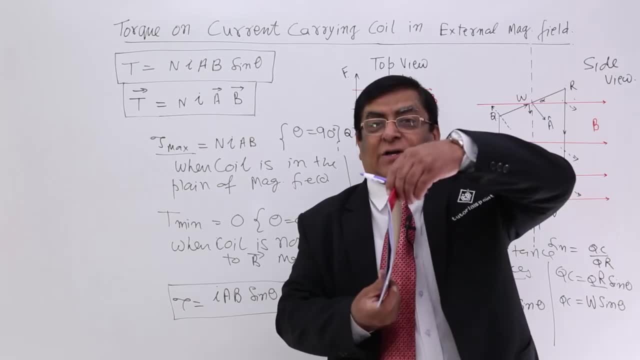 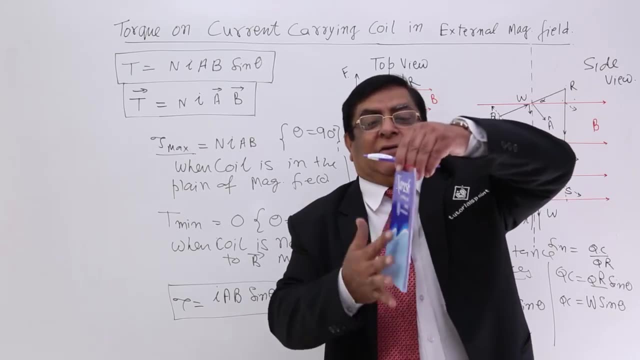 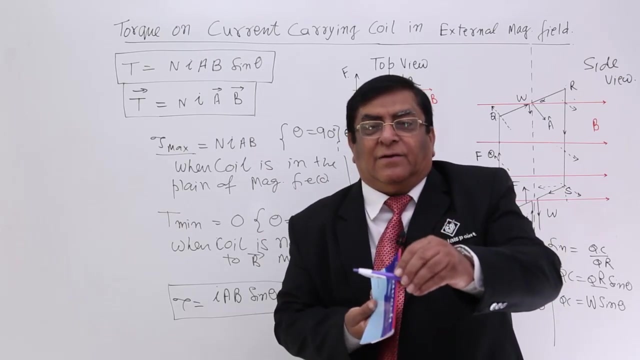 How much is the torque? 0. If this torque is 0, that means what That means: it is not able to rotate, It will not rotate itself and it will stop like this. So if I place a coil perpendicular to it flow current in it, it will not rotate because 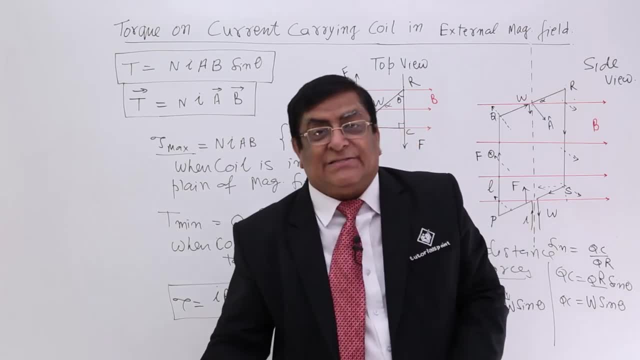 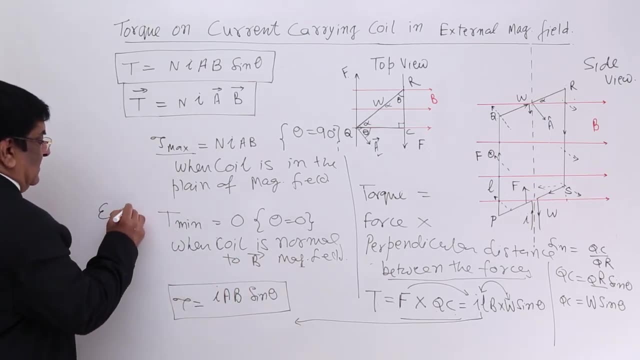 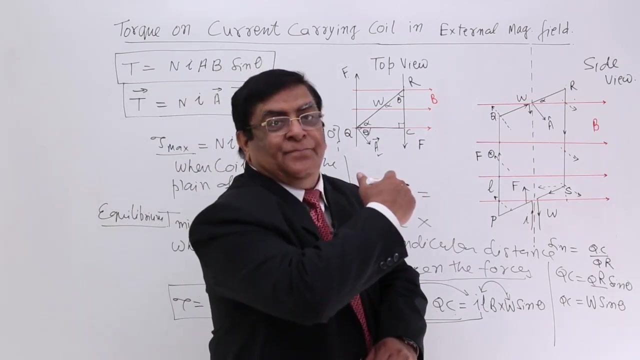 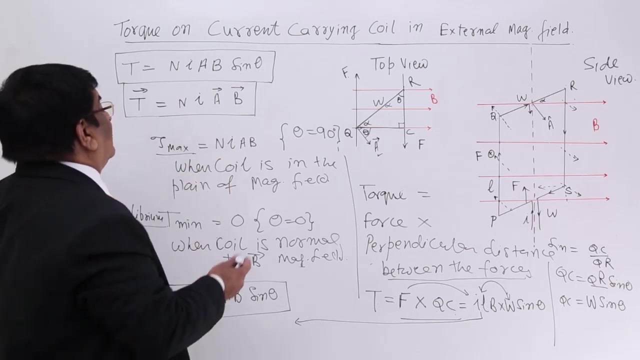 at 90 degree, the torque applicable is 0. So we can also call it equilibrium condition. This is equilibrium. Now, if I rotate it further, 90 degree More, 180 degree, Okay, Make it 180 degree Again. it will become maximum, but the direction will be opposite to that. 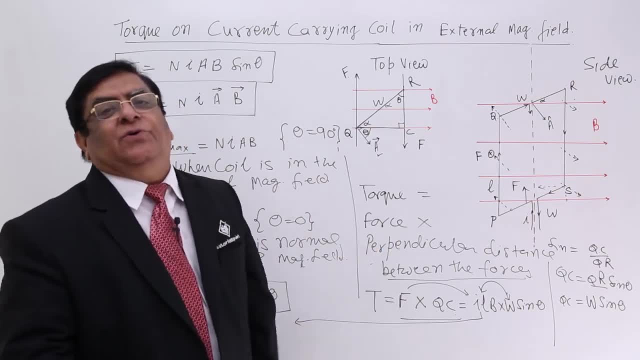 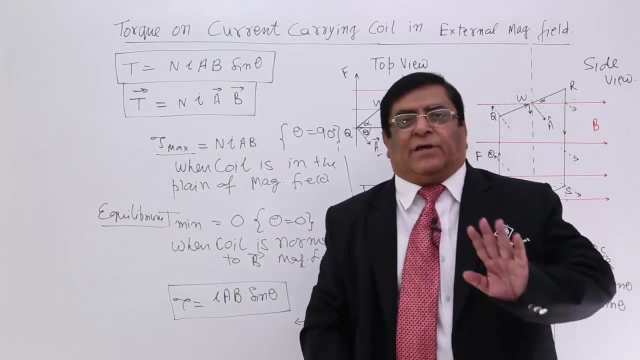 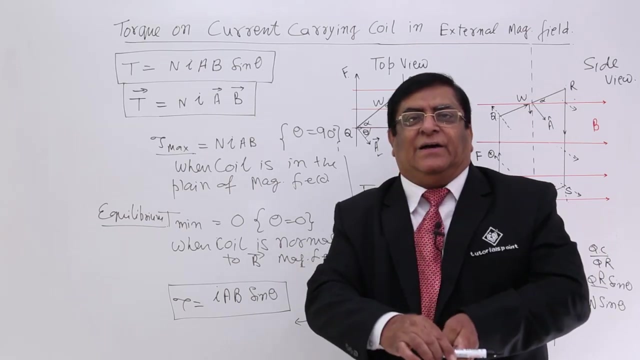 So again, make it 270, it will be 0 again. So this way you can always find out the value of torque. but you should remember the thumb rule: When the coil is in the plane of magnetic field maximum, when it is at right angle. 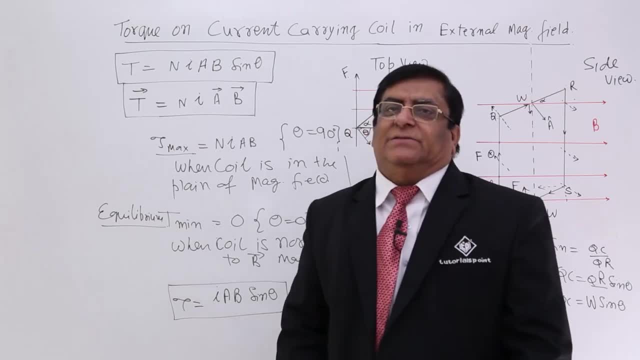 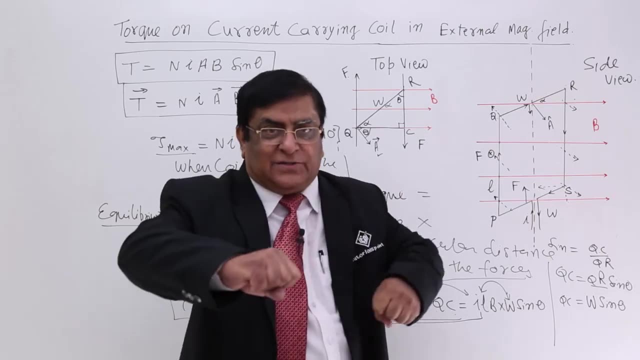 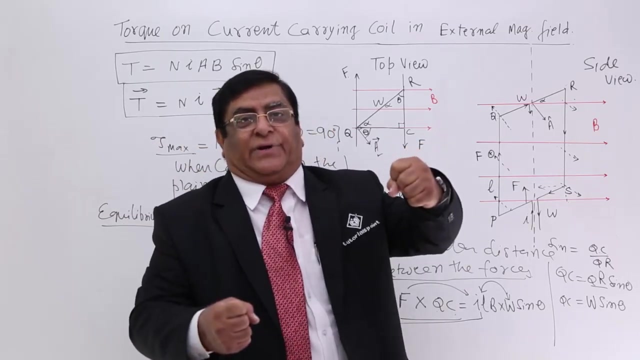 torque is 0.. Okay, So this is torque on a current carrying coil, which is? and what happens with this torque? Answer: when we apply torque on something like a cycle handle, like a steering, it is trying to rotate. It is trying to rotate, it is applying a force, we call it, it is applying a torque and it. 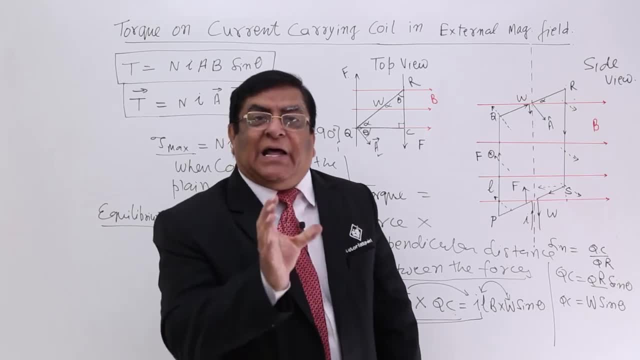 wants to rotate. So unless we stop it, unless we apply a opposite torque, it will rotate. When we apply torque on a wheel, the wheel rotates. So this is torque on a current carrying coil. And what happens with this torque? The wheel rotates. 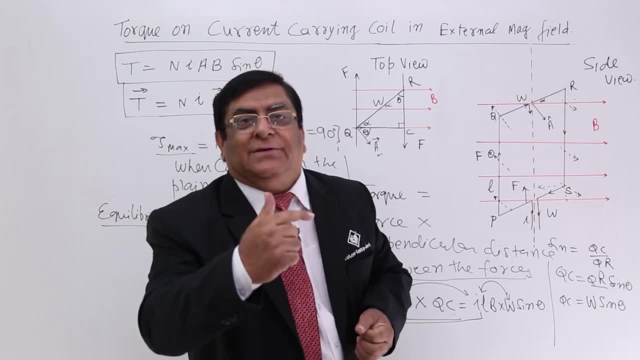 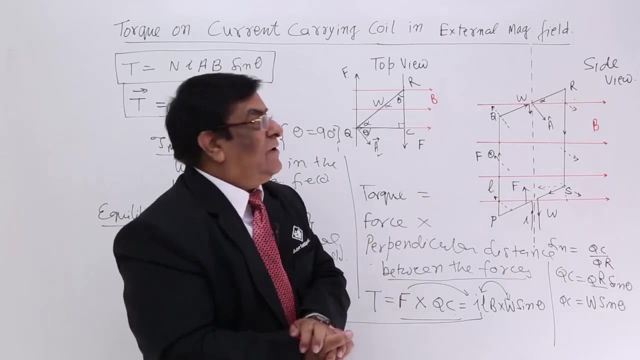 But when we apply an anti-torque with the help of a brake, then the two torques opposite to each other, they balance each other. the wheel stops Okay. So this is torque due to current. Thank you.